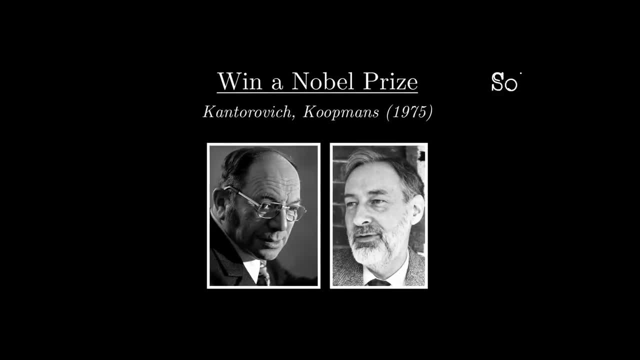 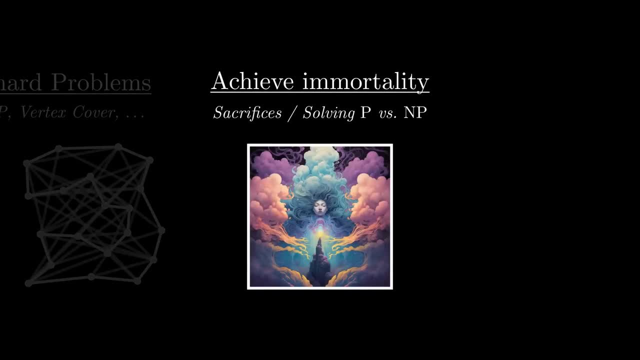 Would you like to win a Nobel Prize in Economics, Or be able to formulate and solve NP-hard problems in an efficient way, Or perhaps transcend the mortal plane and achieve eternal life? Well, in this video I'll cover the first two, the third being left as an exercise for the reader. 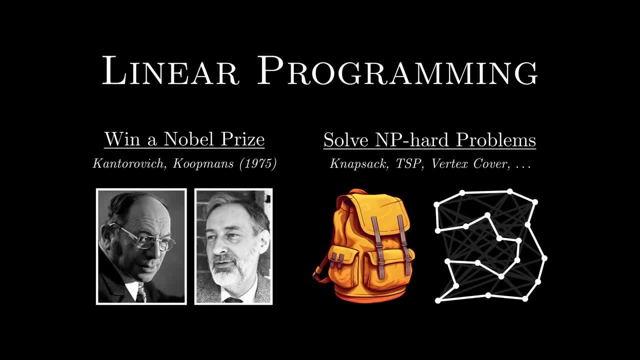 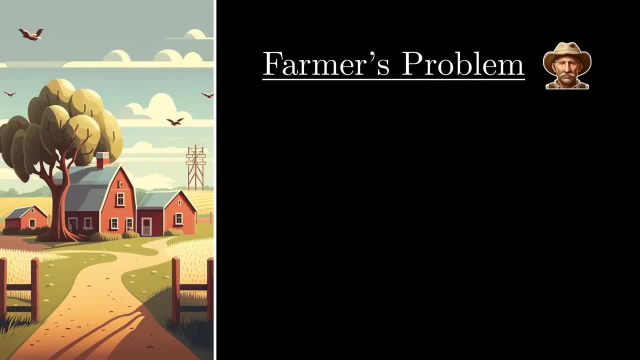 since they both utilize the powerful technique of linear programming. To see what it's all about, let's start with a simple problem. With the planting season steadily approaching, your farmer friend presents you with the following task: You have 3 tons of potato seeds and 4 tons of carrot seeds To grow the crop sufficiently. 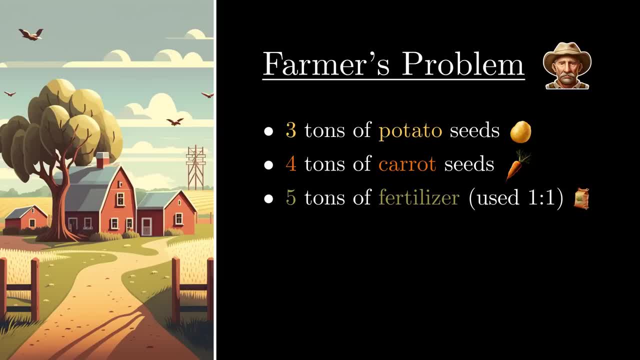 you also have 5 tons of fertilizer which has to be used when planting. in a one-to-one ratio, ie 1 kilogram of potato or carrot seeds requires 1 kilogram of fertilizer. The profit is $1.2 per kilogram for potato seeds and $1.7 per kilogram for carrot seeds. 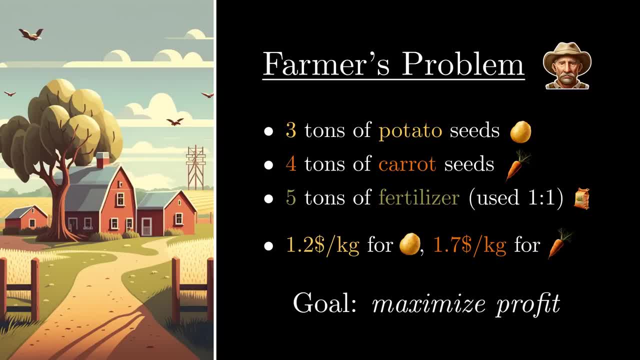 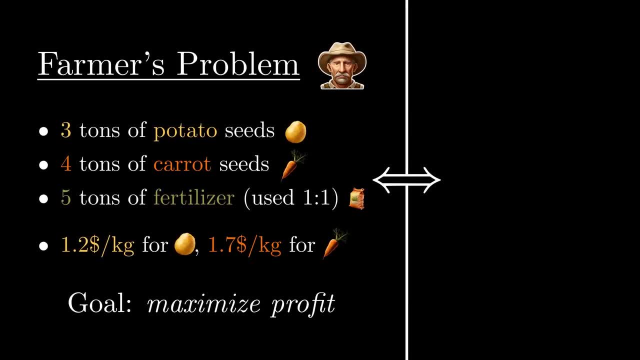 Your goal is to maximize your profit this season. How much potatoes and carrots should you plant? To solve this problem, let's first formalize it. We'll start by creating variables- xp and xc- for the amount of potatoes and carrots planted in kilograms. Both are non-negative real numbers, since planting a negative amount of seeds is. 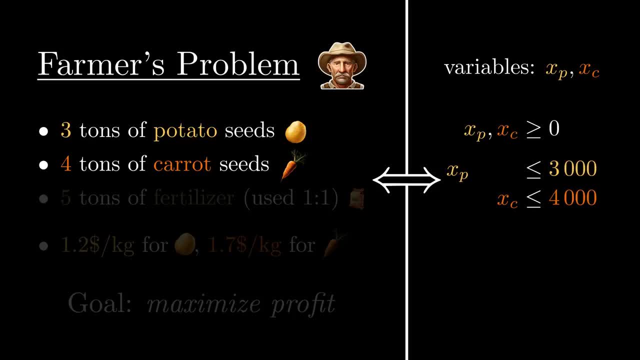 difficult and are bounded by the amount we have. Additionally, their sum is bounded by the amount of fertilizer we have, since it has to be used in a one-to-one ratio for both potatoes and carrots. The profit can then be calculated by the number of potatoes and carrots planted. 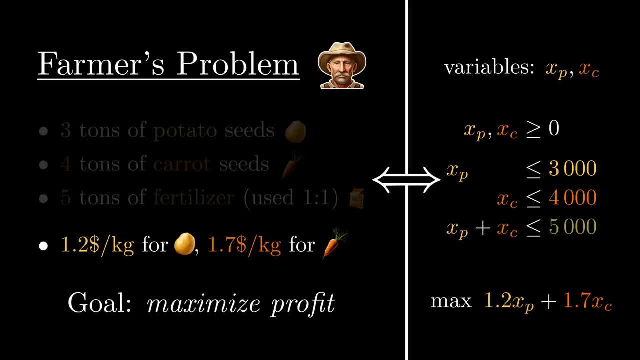 The profit can then be described as 1.2xp plus 1.7xc, and we'll call it the objective function, since it's the function we're trying to maximize. Now that the problem is formalized, it might be helpful to visualize it. 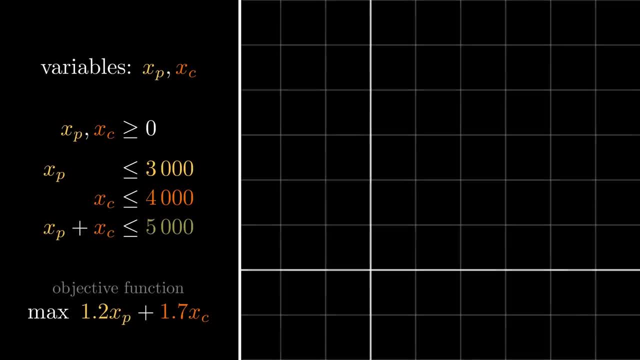 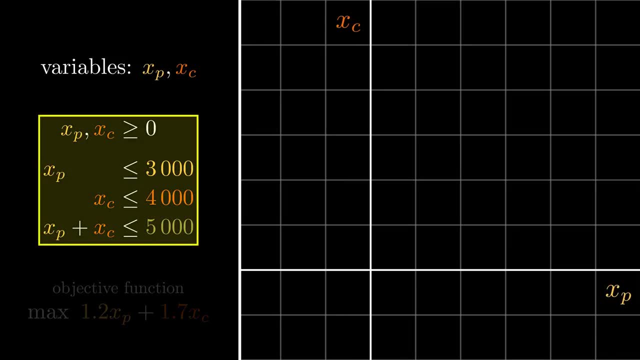 Since we have two variables, it's probably a good idea to use a plane with one axis for each To display the inequalities. we can notice that they are all linear, which means that they are just a weight sum of the variables and each one defines a line with. 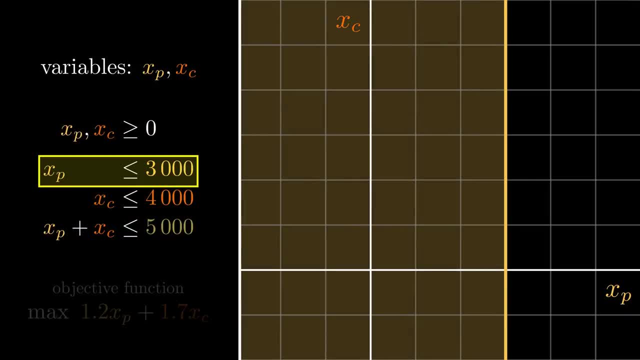 valid values on one side, Therefore they are all linear. So the solution is to use these values on one side- a half-plane to be exact- To satisfy all of the inequalities. we're interested in the intersection of these half-planes, which is the following: 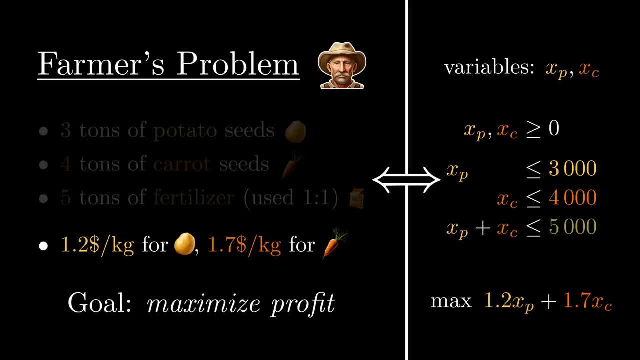 The profit can then be described as 1.2xp plus 1.7xc, and we'll call it the objective function, since it's the function we're trying to maximize. Now that the problem is formalized, it might be helpful to visualize it. 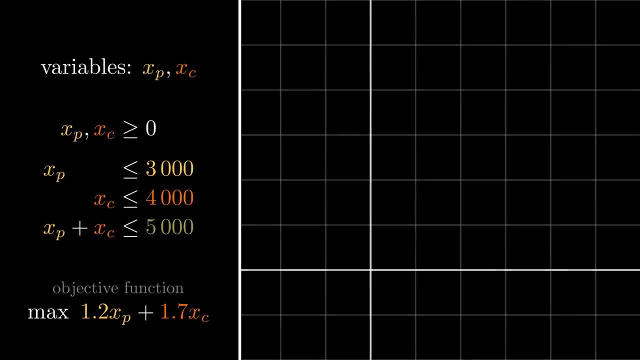 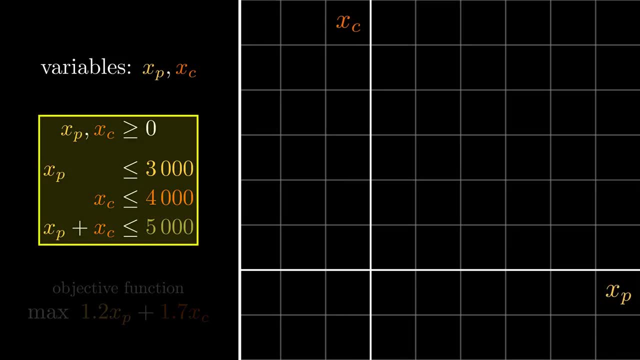 Since we have two variables, it's probably a good idea to use a plane with one axis for each To display the inequalities. we can notice that they are all linear, which means that they are just a weight sum of the variables and each one defines a line with valid. 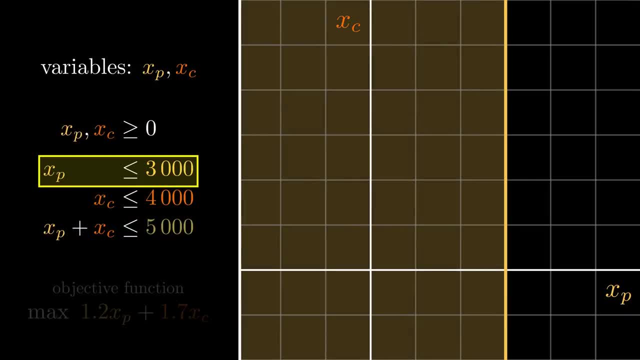 values on one side. This means that the variables are just a weight sum of the variables and each one defines a line with valid values on one side, A half-plane to be exact, To satisfy all of the inequalities. we're interested in the intersection of these half-planes. 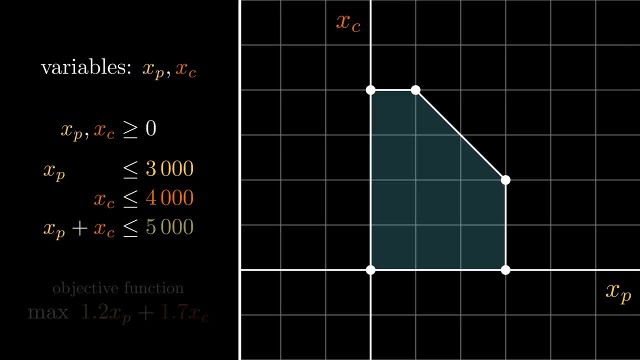 which is the following region. This is pretty useful, since we now know that any solution to our problem will be contained here. But our main task is to maximize the objective function. Pause here and see if you can figure out what it means geometrically in terms of this visualization. 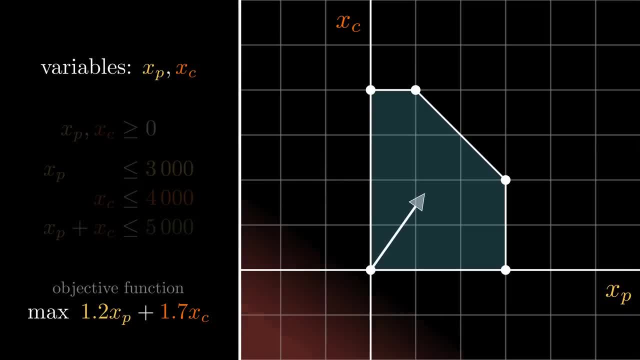 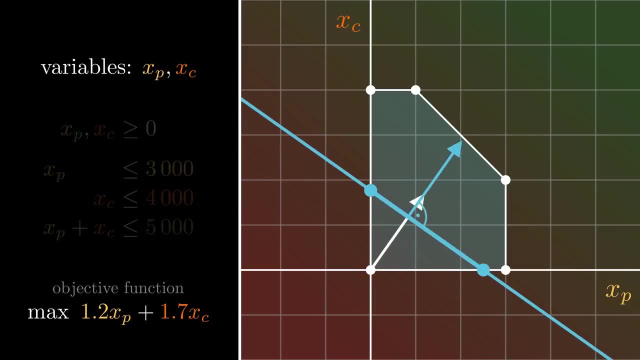 Since the objective function is also linear, it defines a direction in which its value increases. To solve the problem, all we then have to do is move in this direction and record the last intersection, which is the optimum In our case, 1,000 kilograms of potato seeds and 4,000 kilograms of carrot seeds. 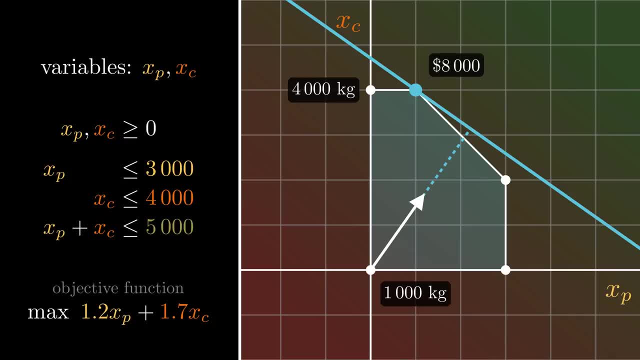 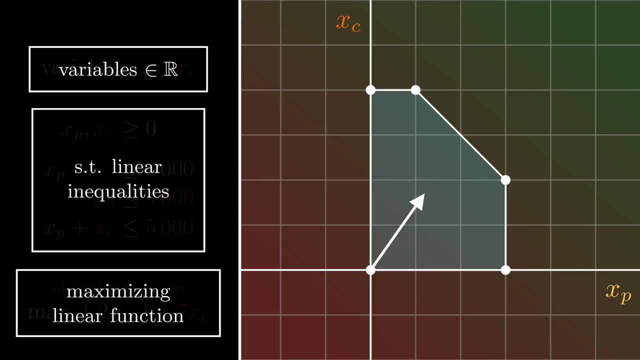 bringing the total profit to 8,000 dollars And, surprisingly, that's all there is to linear programming. We want to find the value of real variables that are subject to linear inequalities and that maximize a linear function. This is a pretty simple example, but a linear program can be much more complex. 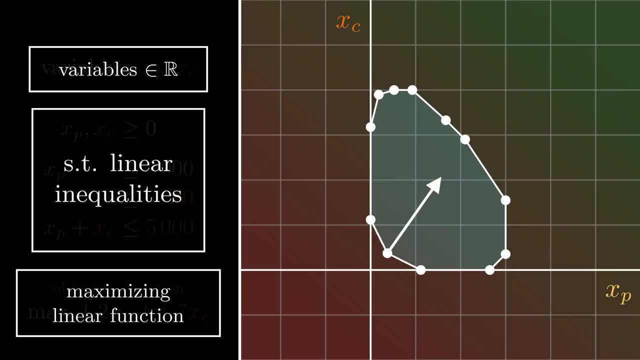 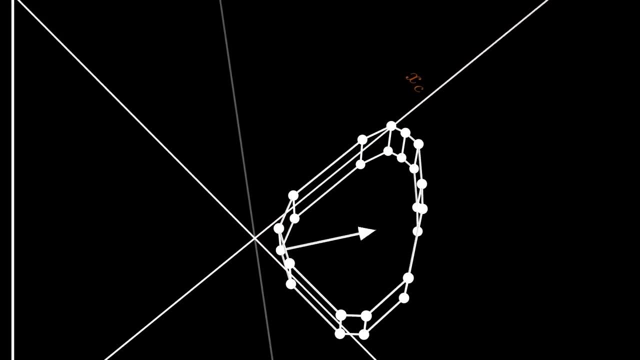 It can contain any number of inequalities which complicate the shape of our region and also any number of variables which bring us from 2D for two variables to 3D for three and beyond. So while the general concept stays the same, our simpler geometric solution won't. 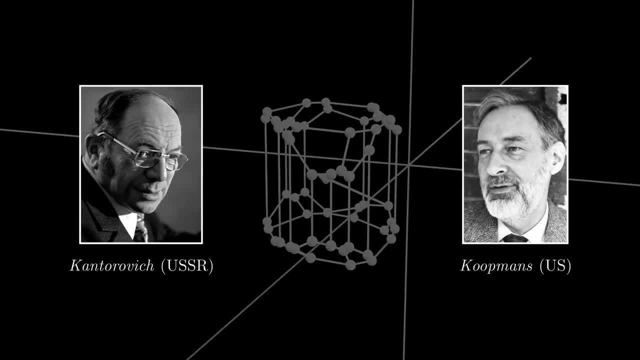 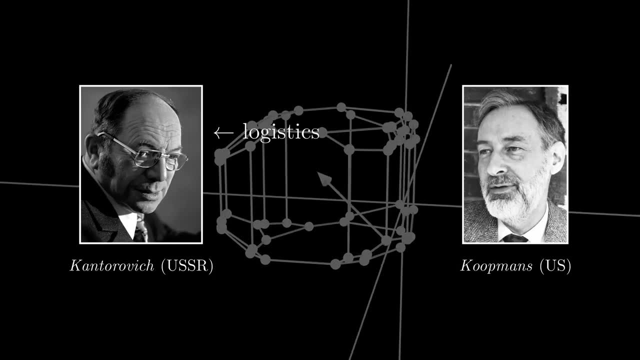 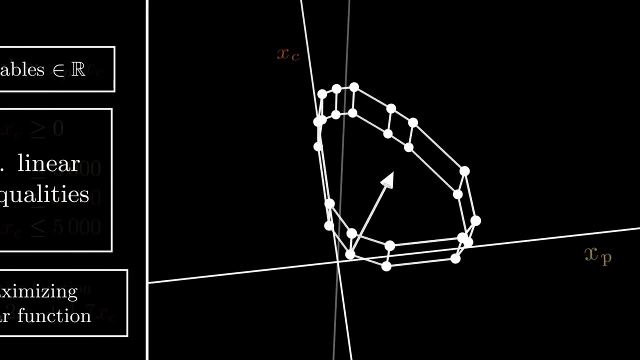 do for larger programs. The Nobel Prize I mentioned at the beginning of the video was awarded to Kantorowicz and Koopmans in 1975 for formulating a number of classic logistics and economics problems in this model, which are again too complicated to be solved geometrically. So instead, 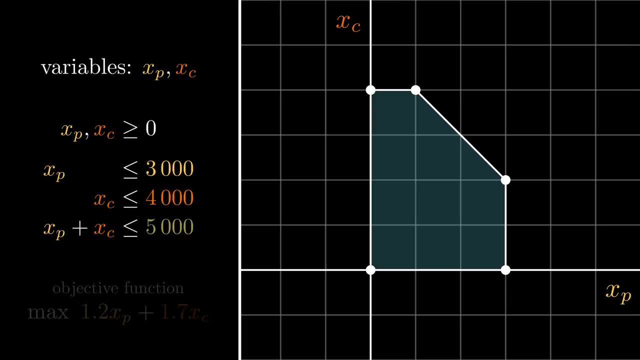 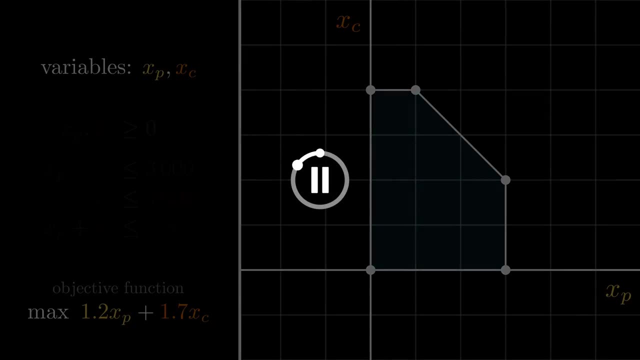 region. This is pretty useful, since we now know that any solution to our problem will be contained here. but our main task is to maximize the objective function. Pause here and see if you can figure out what it means geometrically in terms of this visualization. 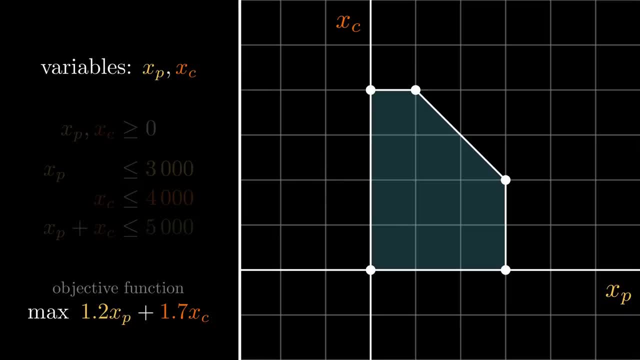 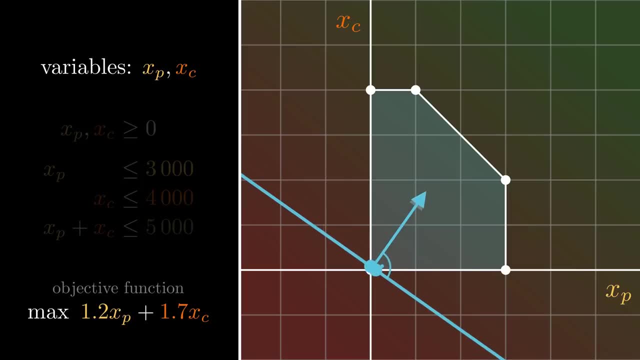 Since the objective function is also linear, it defines a direction in which its value increases. To solve the problem, all we then have to do is move in this direction and record the last intersection, which is the optimum. In our case, 1,000 kilograms of potato seeds and 4,000 kilograms of. 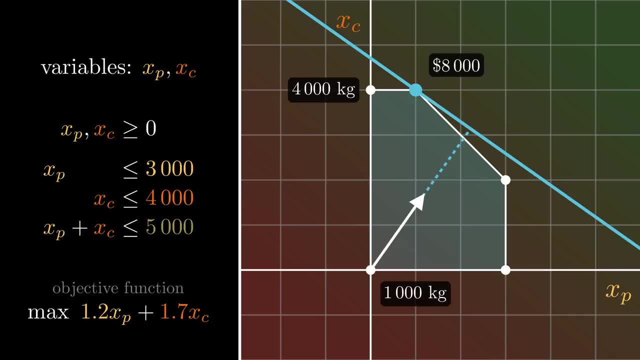 carrot seeds, bringing the total profit to $8,000.. And surprisingly, that's all there is to linear programming. We want to find the value of real linear programming. We want to find the value of real variables that are subject to linear inequalities and that maximize a linear 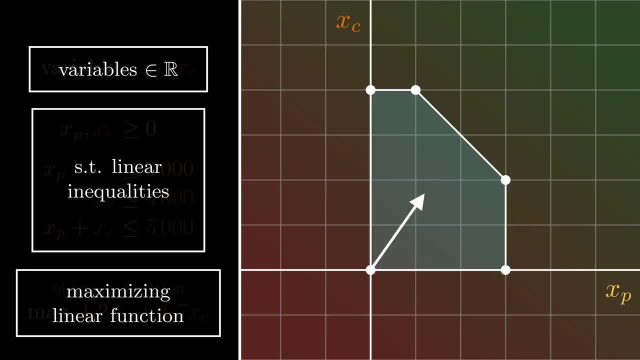 function. This is a pretty simple example, but a linear program can be much more complex. It can contain any number of inequalities which complicate the shape of our region and also any number of variables which bring us from 2D for two. 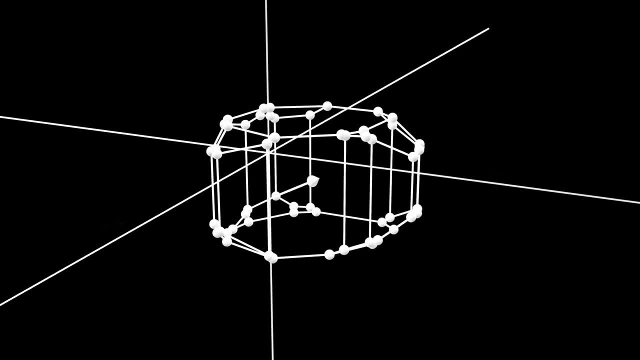 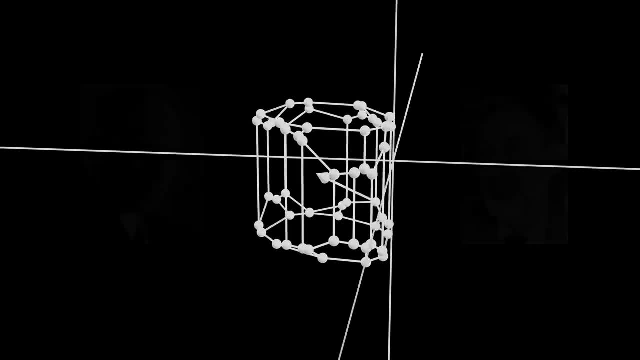 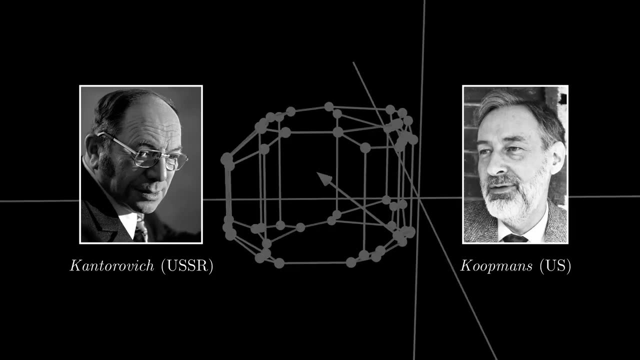 variables to 3D for three and beyond. So while the general concept stays the same, our simpler geometric solution won't do for larger programs. The Nobel Prize I mentioned at the beginning of the video was awarded to Kantorowicz and Koopmans in 1975 for formulating a number of classic. 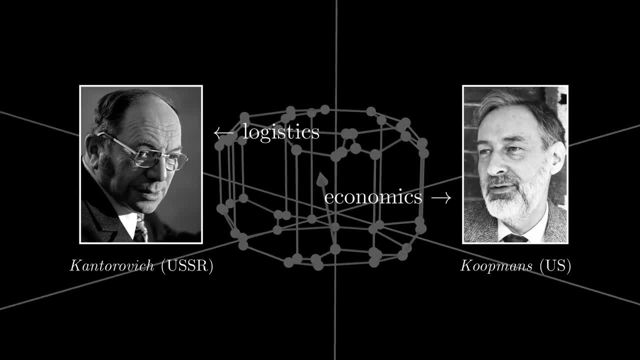 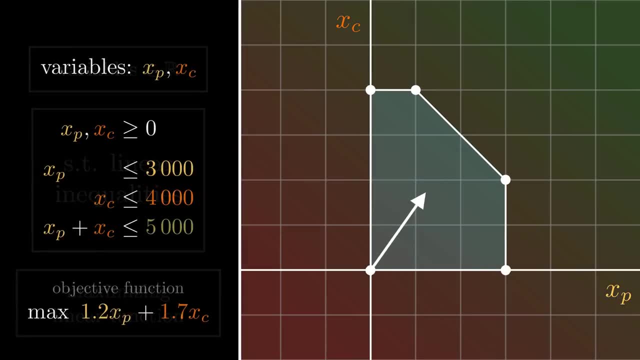 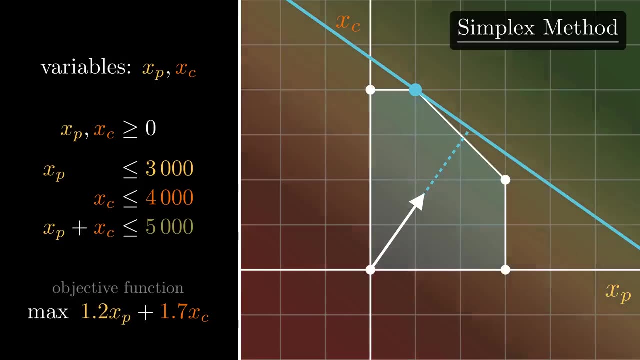 logistics and economics problems in this model, which are again too complicated to be solved geometrically. So instead let's look at how to solve a linear program algorithmically using the simplex method, Similar to the geometric solution. we will again be moving in the direction of the objective function, but 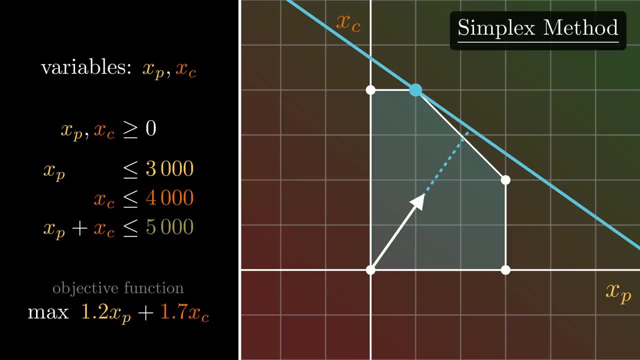 we'll do so in a smarter way. For this we'll use the fact that the optimum will be achieved in at least one vertex. It can sometimes be more like a whole line, but some vertex will still achieve it, as we see, by doing a full rotation. This means that we can move from vertex to vertex which. 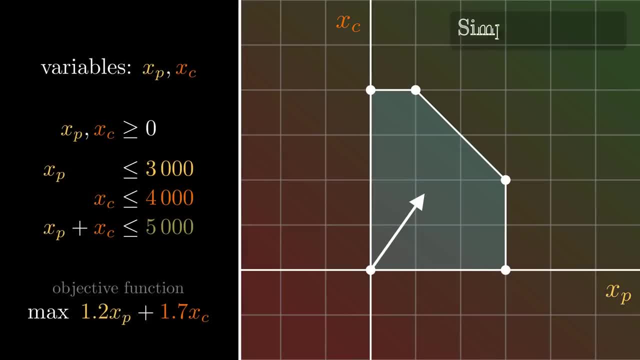 let's look at how to solve a linear program algorithmically using the simplex method, Similar to the geometric solution. we will again be moving in the direction of the objective function, but we'll do so in a smarter way. For this we'll use the fact that the optimum will be achieved in at least one vertex. 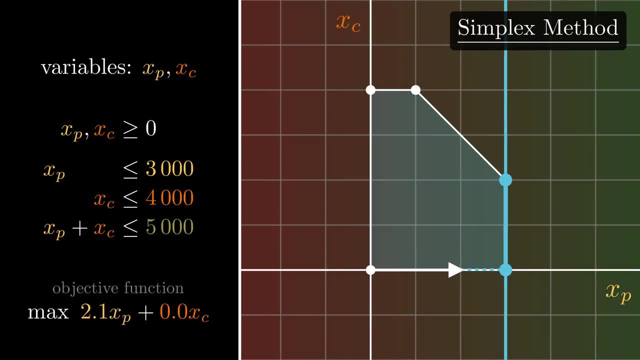 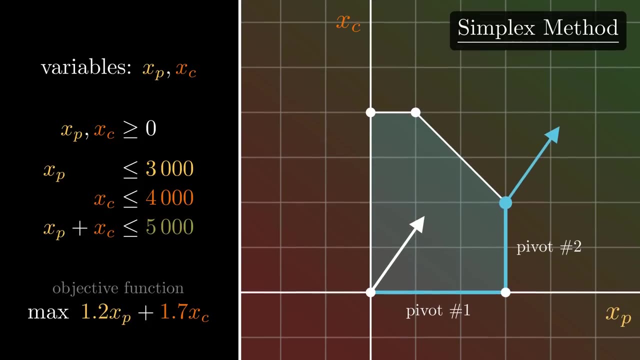 It can sometimes be more like a whole line, but some vertex will still achieve it, as we see, by doing a full rotation. This means that we can move from vertex to vertex- which is called pivoting- always picking one that brings us closer to our goal, Until we can't any longer, at which point we know we found the optimum. 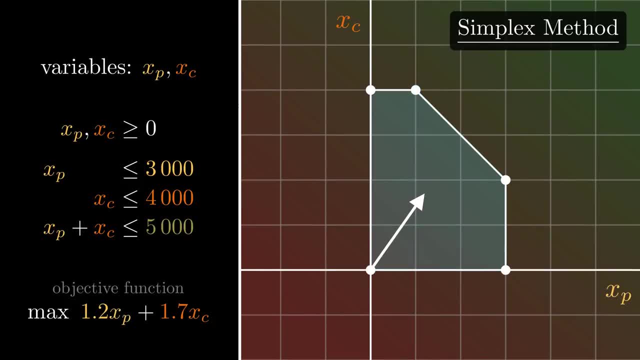 But before I get into that, let me show you how to use a linear function to solve the problem in a simpler way. I tell you how it works. let me tell you a short story. It's 1939 and a student of mathematics- 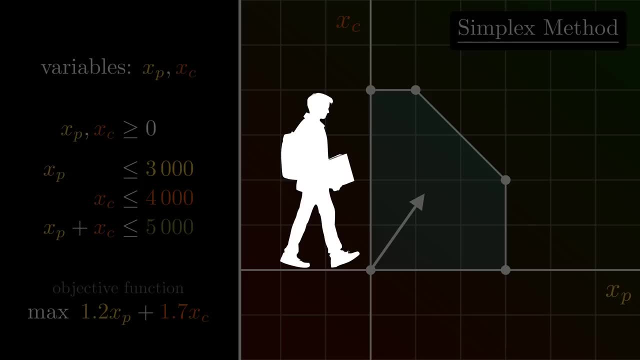 arrives late to a lecture, He sees two problems on the board and, assuming they are homework, writes them down. They prove to be more challenging than usual, but he perseveres and hands them back a week later with an apology that they took him so long. 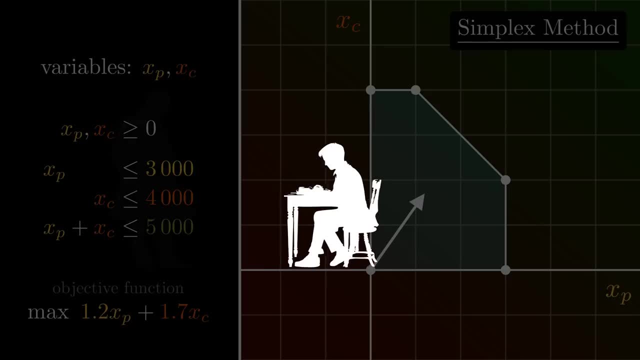 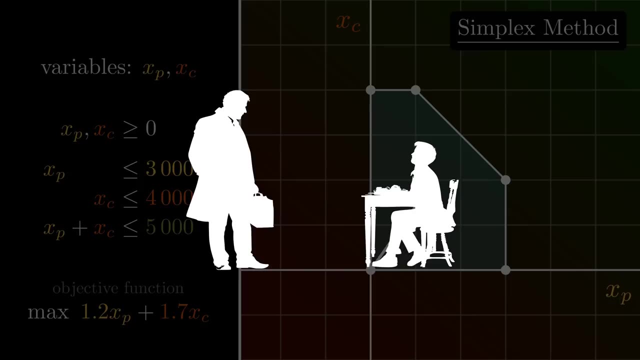 A few weeks go by and the student is surprised by a knock on the door by the professor himself, who reveals to him that they were two famous unsolved problems in the field of statistics. You might have heard this story or a version of it, since it's an urban legend in the mathematical 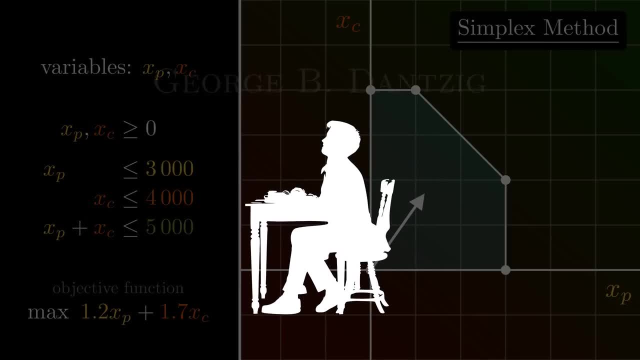 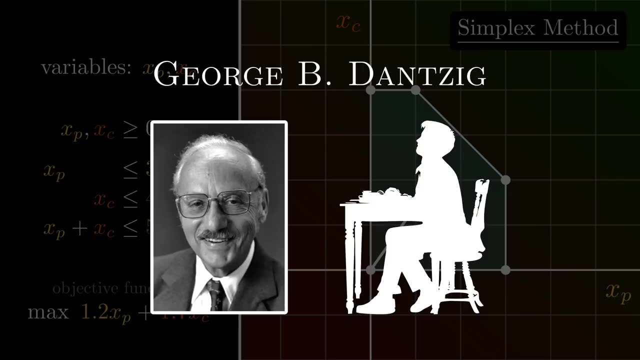 world, but what you might not know is that the student was George B Danzig, the inventor of the algorithm I just described. I stumbled upon this story about Danzig and many more when doing research for this video and it was too good to exclude, so if there's something you should take. 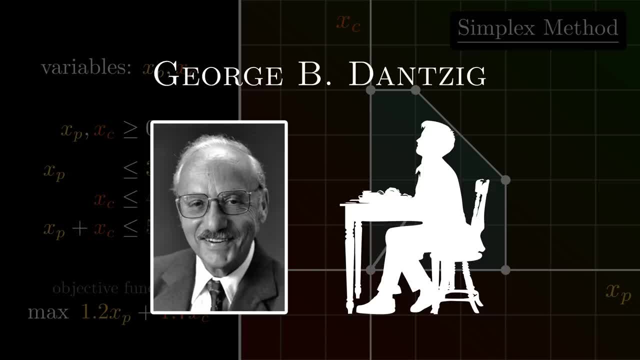 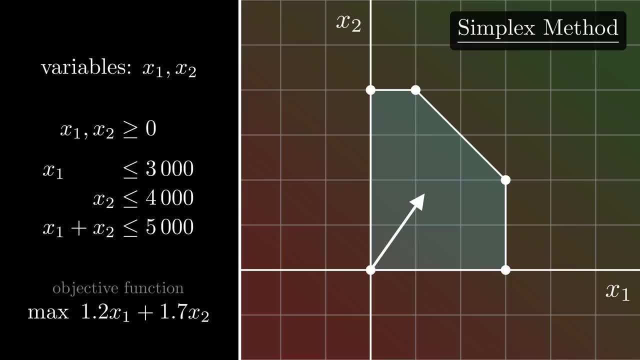 away. it's that George B Danzig was a really cool guy. Getting back to the topic at hand, we'll first rename the variables to x1 and x2, which is the standard way of naming variables in a linear program. To understand how pivoting works numerically, let's consider what happens when we're in a vertex. 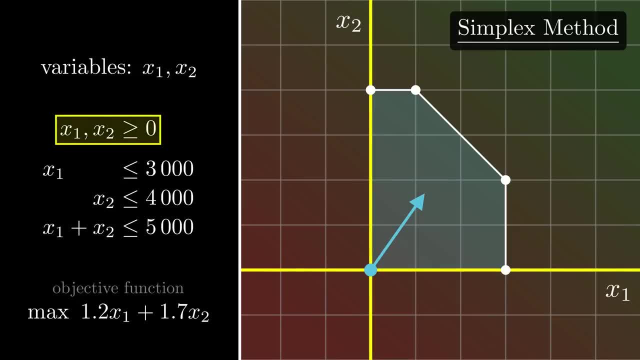 Taking 0,0 as an example, we see that two of the inequalities are tight, which means that the left side is equal to the right side in this case, because both x1 and x2 are zero. Now say we want to pivot from this vertex to an adjacent one. 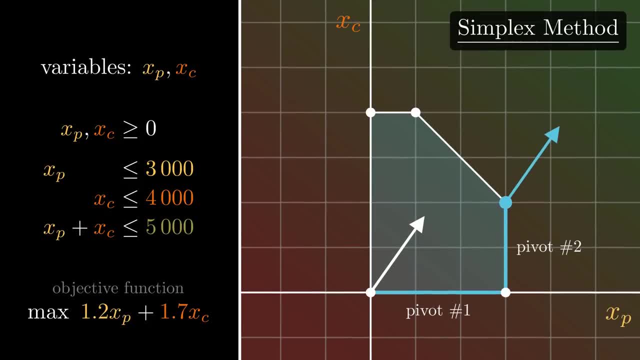 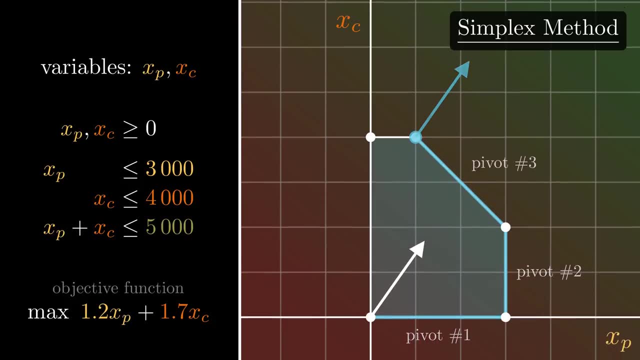 is called pivoting, always picking one that brings us closer to our goal Until we can't any longer, at which point we know we've found the optimum. But before I tell you how it works, let me tell you a short story. It's 1939 and a student of mathematics 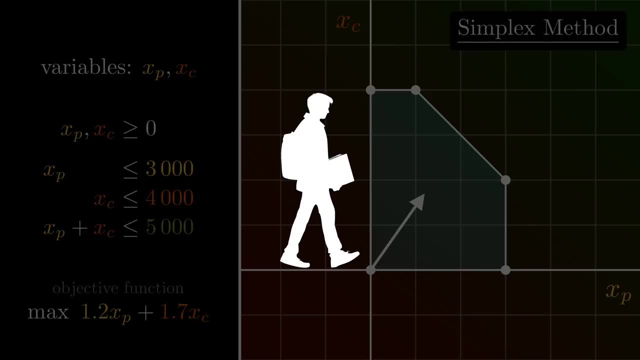 arrives late to a lecture, He sees two problems on the board and, assuming they are homework, writes them down. They prove to be more challenging than usual, but he perseveres and hands them back a week later with an apology that they took him so long. A few weeks go by and the student is surprised by a knock on. 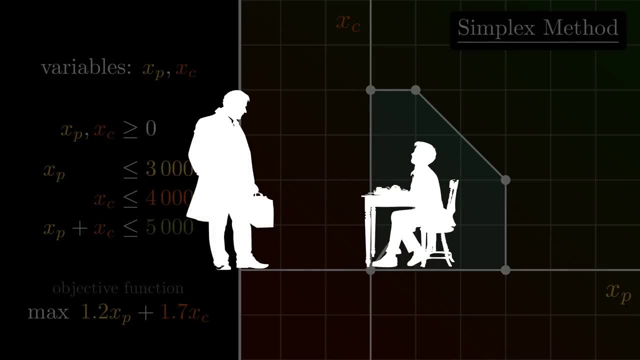 the door by the professor himself, who reveals to him that they were two famous unsolved problems in the field of statistics. You might have heard this story, or a version of it, since it's an urban legend in the mathematical world, but what you might not know is that the student was George B Danzig. 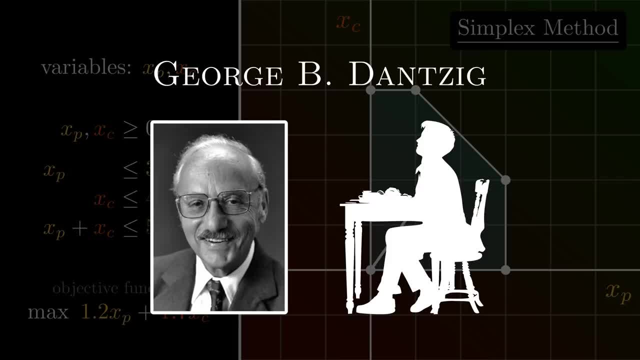 the inventor of the algorithm I just described. I stumbled upon this story about Danzig and many more when doing research for this video, and it was too good to exclude. so if there's something you should take away, it's that George B Danzig was a really cool guy. 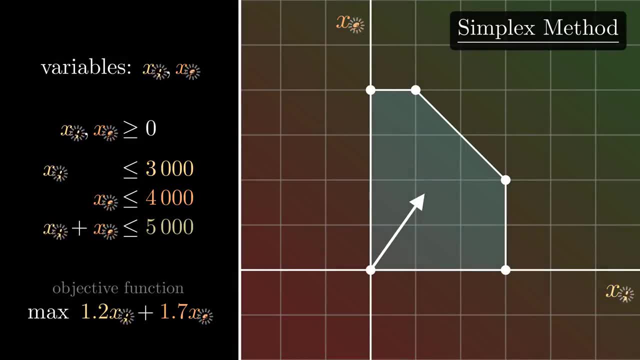 Getting back to the topic at hand, we'll first rename the variable to x1 and x2, which is the standard way of naming variables in a linear program. To understand how pivoting works numerically, let's consider what happens when we're in a vertex. Taking 0, 0 as an example, we see that two of the 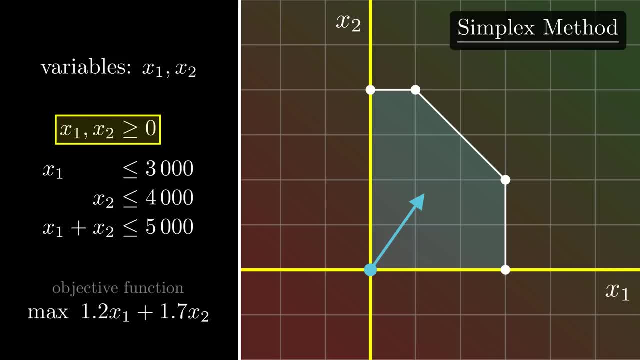 inequalities are tight, which means that the left side is equal to the right side in this case, because both x1 and x2 are 0. Now say we want to pivot from this vertex to an adjacent one. To perform this pivot, we first have to loosen one. 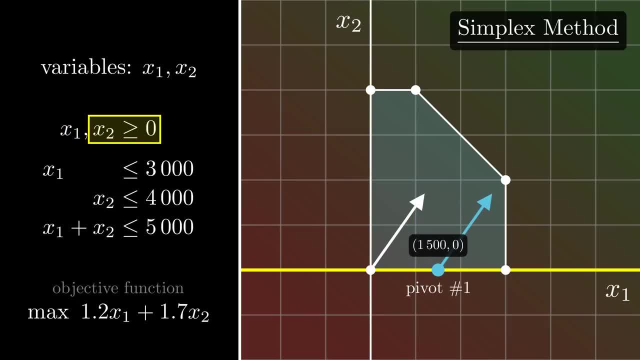 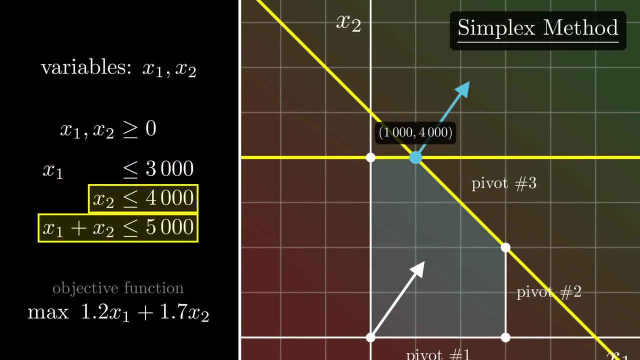 inequality, which determines the direction we move in, and tighten another, which determines how far we go. This is the crucial idea behind the simplex algorithm: Loosen one and tighten another until we reach the optimum In order to calculate which variables to loosen. 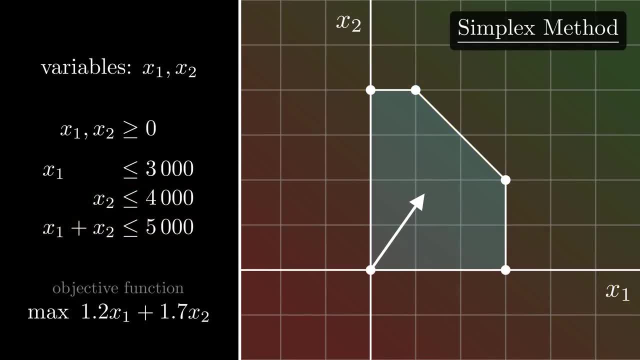 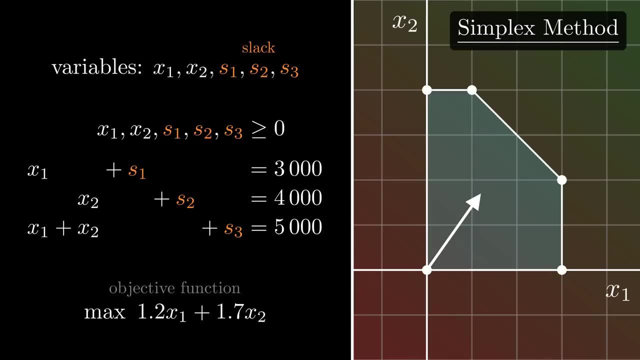 and which to tighten. we'll slightly modify our program to make the math easier. We'll introduce new variables for each inequality, called slack variables, which act as the difference between the left and the right side, thus turning the inequalities into equalities. This means that a tight inequality before is the same as a variable being set. 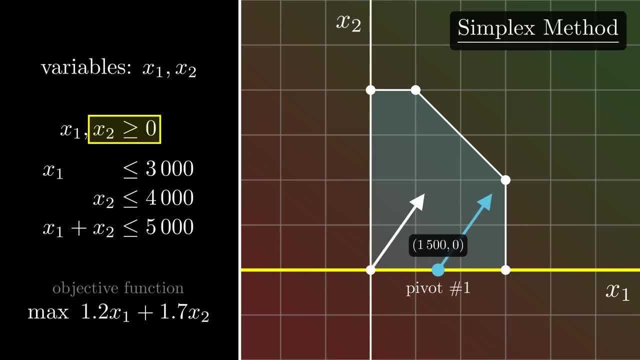 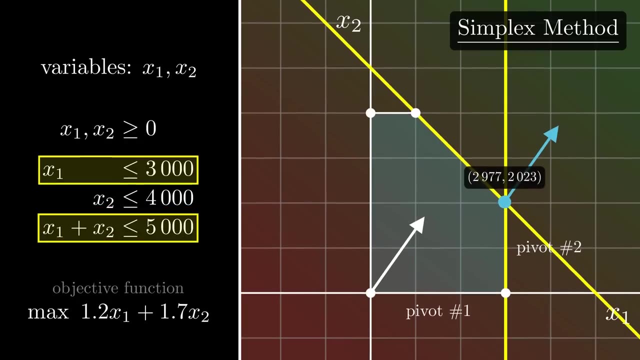 To perform this pivot, we first have to loosen one inequality, which determines the direction we move in, and tighten another, which determines how far we go. This is the crucial idea behind the simplex algorithm: Loosen one and tighten another until we reach the optimum. 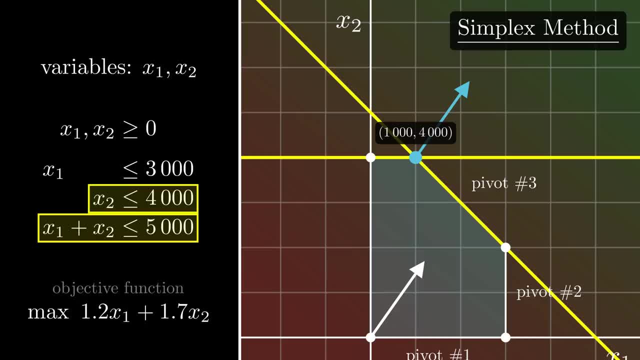 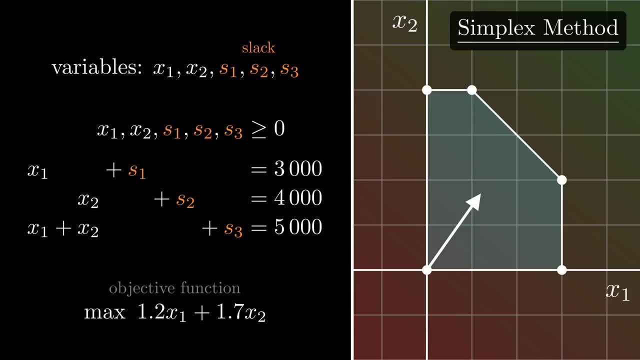 In order to calculate which variables to loosen and which to tighten, we'll slightly modify our program to make the math easier. We'll introduce new variables for each inequality, called slack variables, which act as the difference between the left and the right side, thus turning the inequalities into equalities. This means that a tight inequality 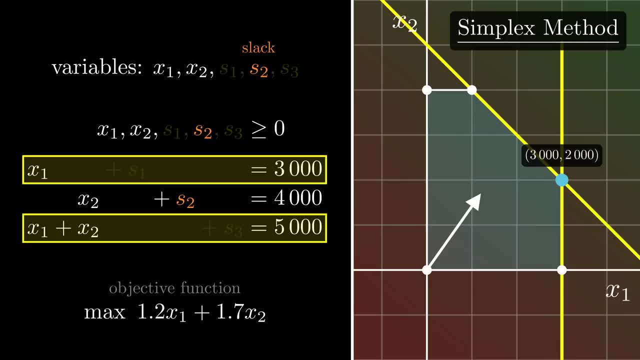 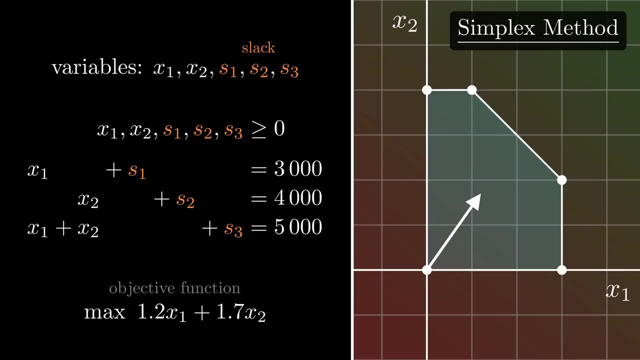 before is the same as a variable being set to zero. now, As you see, since s1 and s3 are zero, the first and third equalities become tight. Feel free to pause here for a second and make sure that this transformation makes sense to you. Let's now get to the actual computation. 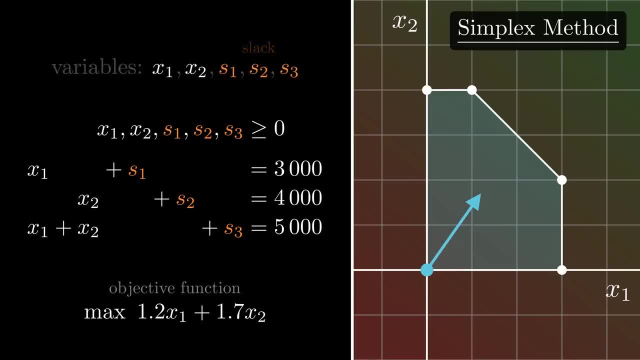 We again start in, which means that the initial tight variables will be x1 and x2.. The tight variables are usually called non-basic and the loose are called basic, But we'll stick with tight and loose for now, since that's what they geometrically mean. 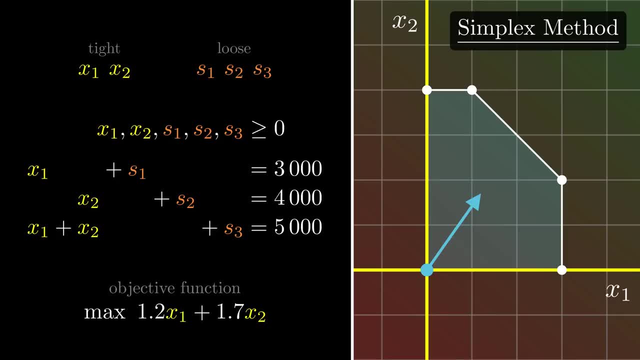 Before we start the first pivot, we'll do two things. First, we'll hide the positive inequalities. They still apply, mind you, but we don't need them for the actual computation, so there is no point in keeping them on the screen. 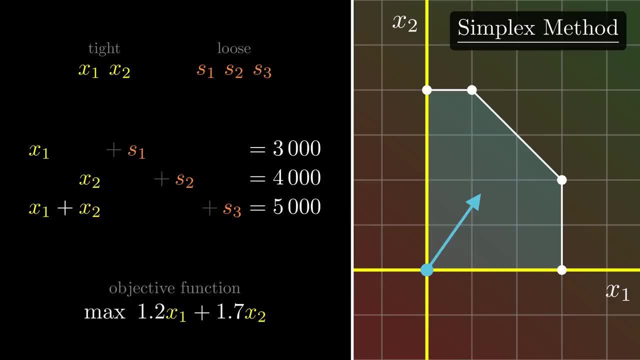 Second, we'll further rewrite the equalities such that the left side only contains loose variables with a coefficient of one. This makes calculating the current solution trivial, since we can just set the tight variables to zero and look at the constants. Okay, now we're finally ready for the pivot. First, we need to loosen a variable to determine. 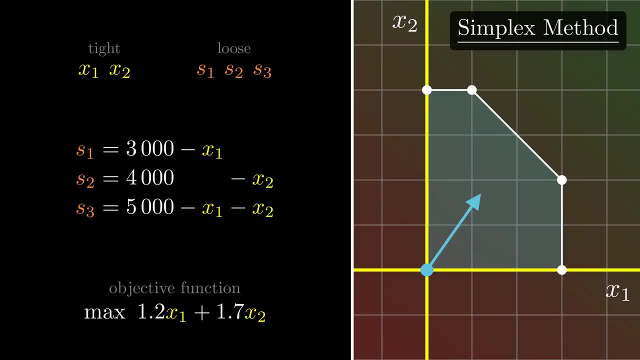 which direction to go. There is a number of methods for selecting which to loosen, but we'll stick with the most commonly used one, called Densig's Pivot Rule, after the inventor himself. The rule is very simple: We select the variable with the largest positive coefficient in the 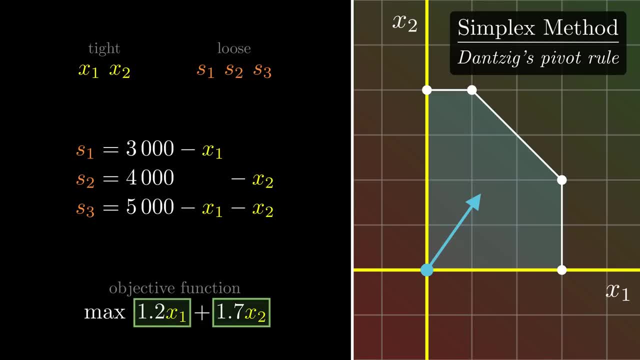 objective function, ie the one representing the steepest direction towards the optimum. In our case, this is x2, which we loosen and start heading in its direction. Now that we've selected the direction to move in, we have to determine how far. 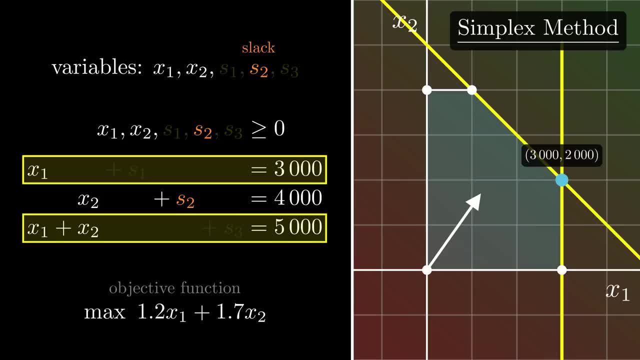 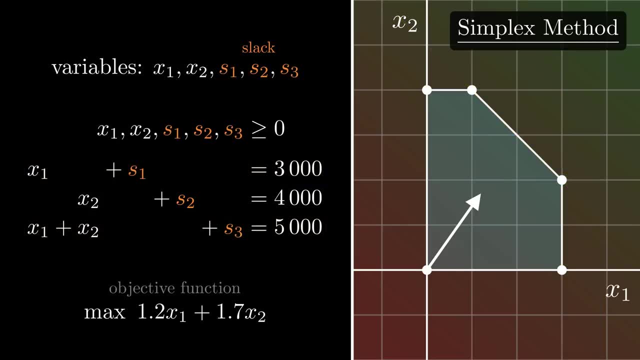 to 0. now, As you see, since s1 and s3 are 0, the first and third equalities become tight. Feel free to pause here for a second and make sure that this transformation makes sense to you. Let's now get to the actual computation. We again start in 0, 0,, which means that the 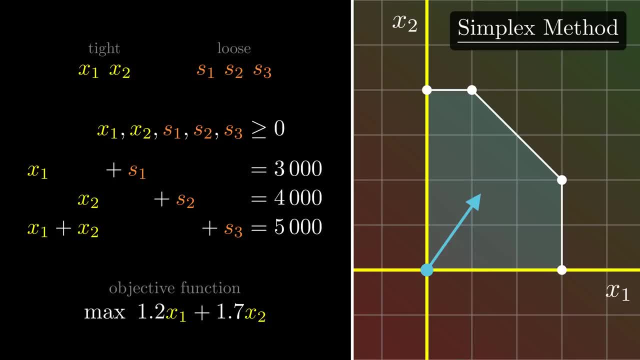 initial tight variables will be x1 and x2.. The tight variables are usually called non-basic and the loose are called basic. but we will stick with tight and loose for now, since that's what they geometrically mean Before we start the first pivot. we'll do two things. First, we will hide the positive. 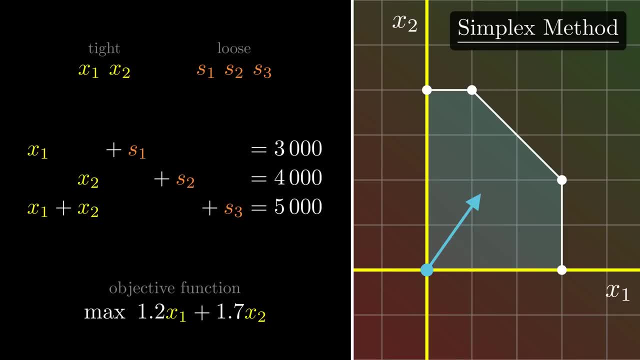 inequalities. They still apply, mind you, but we don't need them for the actual computation, so there is no point in keeping them on the screen. Second, we will further rewrite them when the true revolving the equalities, such that the left side only contains loose variables with a coefficient of 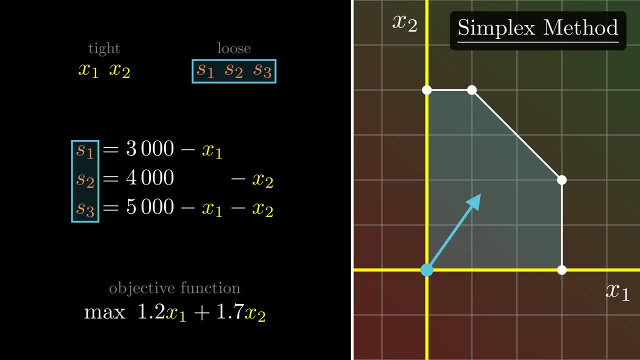 1. This makes calculating the current solution trivial, since we can just set the tight variables to zero and look at the constants. Okay, now we're finally ready for the pivot. First, we need to loosen a variable to determine which direction to go. 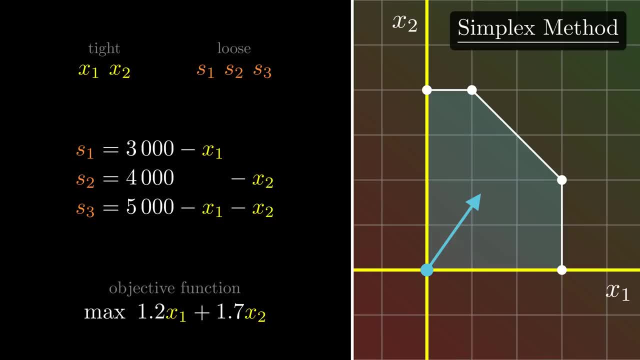 There is a number of methods for selecting which to loosen, but we'll stick with the most commonly used one, called Densik's pivot rule, after the inventor himself. The rule is very simple: We select the variable with the largest positive coefficient in the objective function. 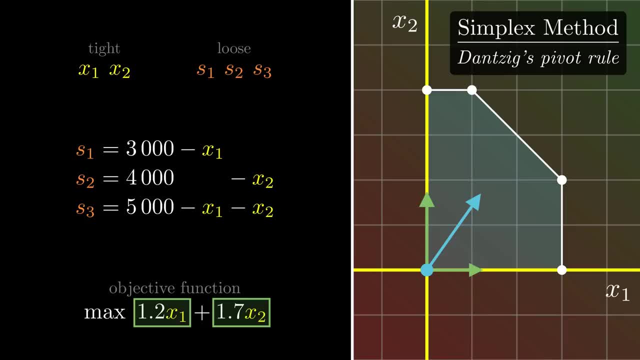 ie the one representing the steepest direction towards the optimum. In our case, this is x2, which we loosen and start heading in its direction. Now that we've selected the direction to move in, we have to determine how far 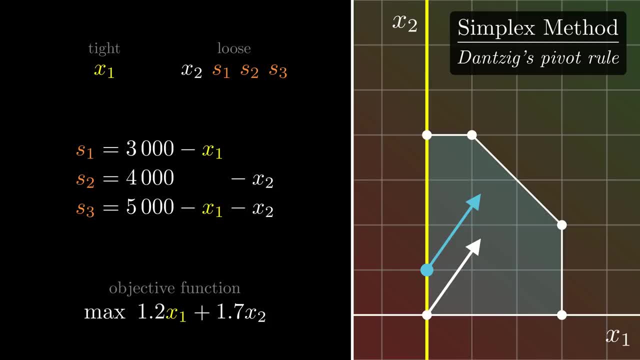 which we'll do by tightening To see what choices we have. we'll look at the equalities where x2 appears, which are s2 and s3, since these are the loose variables constraining it, We want to make either s2 or s3 tight, but as we see, 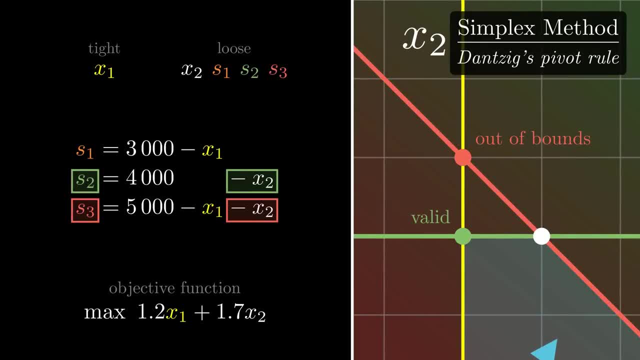 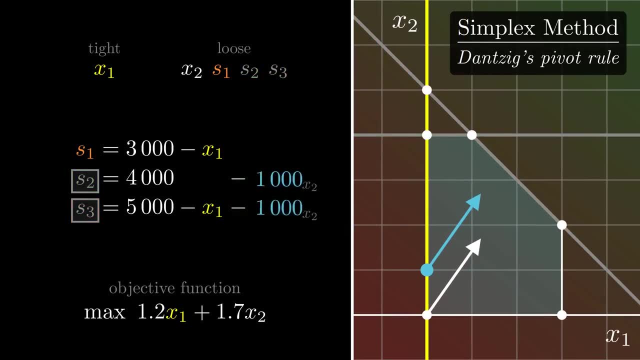 only one of them keeps us in the area of valid solutions. So how can we calculate which one it is? Well, let's simulate what happens when we move in the selected direction. We see that x2 is increasing and its value eventually reaches 4000,. 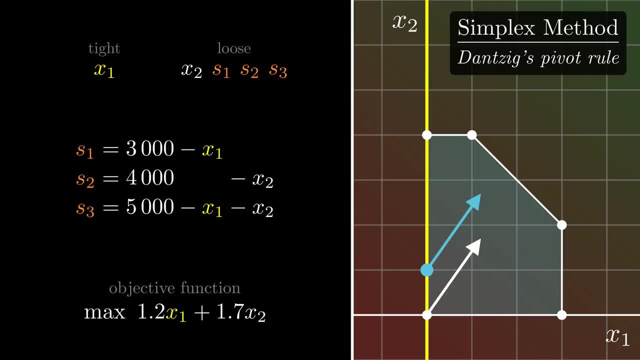 Which we'll do by tightening To see what choices we have. we'll look at equalities where x2 appears, which are s2 and s3, since these are the loose variables constraining it. We want to make either s2 or s3 tight, but, as we see, only one of them keeps us in the 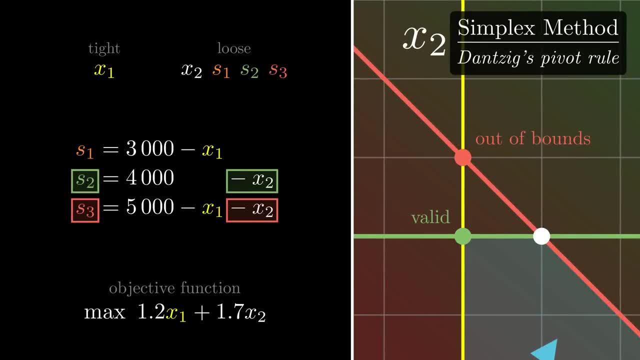 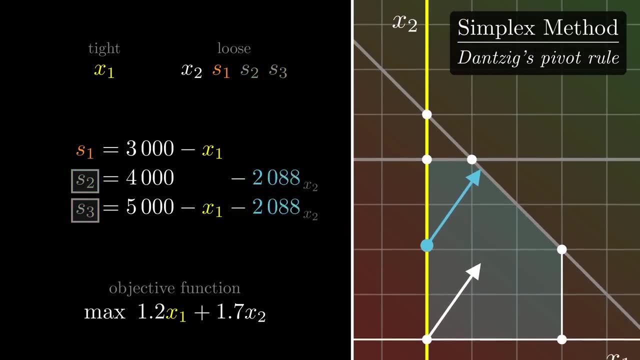 area of valid solutions. So how can we calculate which one it is? Well, let's simulate what happens when we move in the selected direction. We see that x2 is increasing and its value eventually reaches 4000, which evens out the constant value for the second equality. 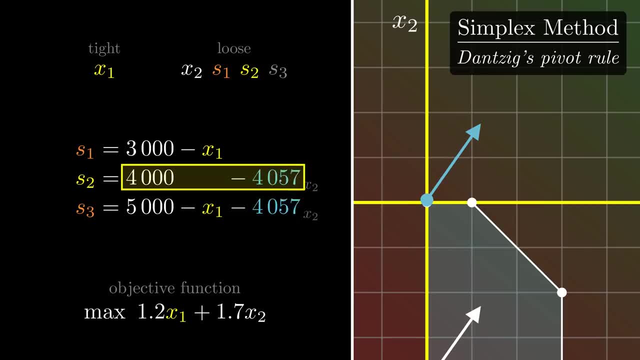 making s2 tight. Now, if we were to go further, s2 would have to go negative for the equality to still work, which is not allowed since all variables have to be non-negative. So in other words, to calculate which variable to tighten, we're interested in the ratio between: 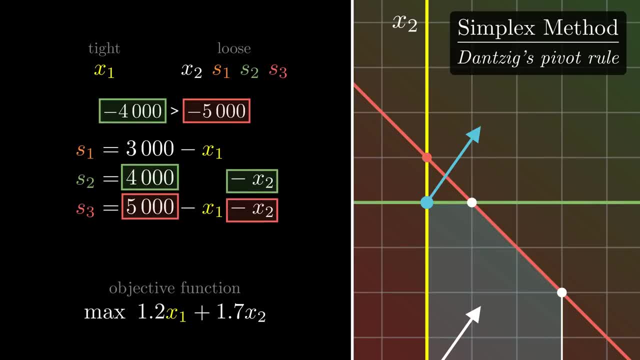 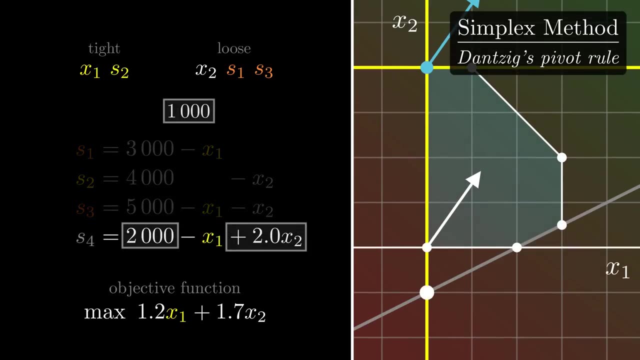 x2 and the constants. The larger it is, the sooner we reach it And, as we've seen, it is indeed s2, which we tighten. Note that if it's greater than zero, for example, if we had another equality like this one, we wouldn't want it, since increasing x2 in this. 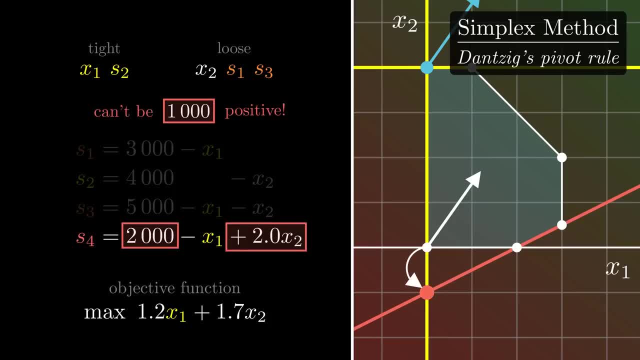 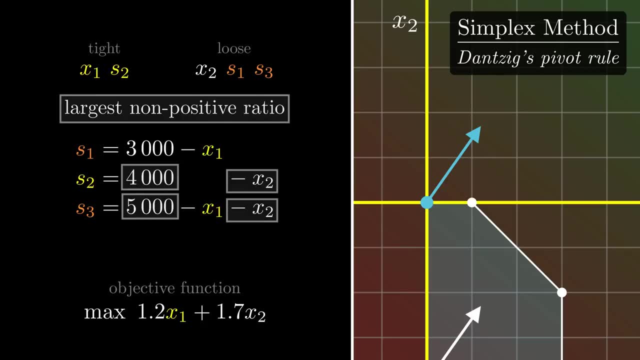 case will never zero out the constant, since it's in the opposite direction. So what we actually want is the largest non-positive ratio. Now that we've loosened x2 and tightened s2,, we still have to fix the equalities and the objective. 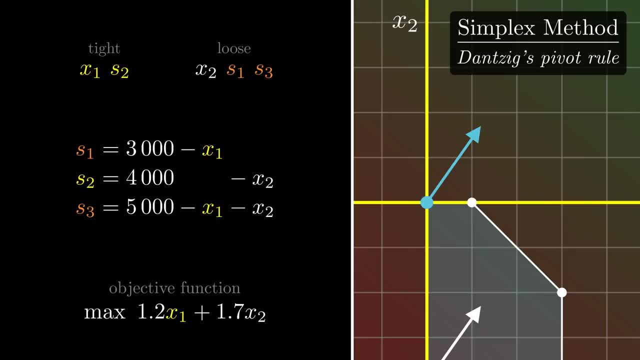 function. Remember that loose variables are not always the same, and that's why we want to make these variables belong only on the left side, which now isn't the case, as you can see by the highlighted s2s and x2s. Swapping them solves the problem. for the second, equality, which we 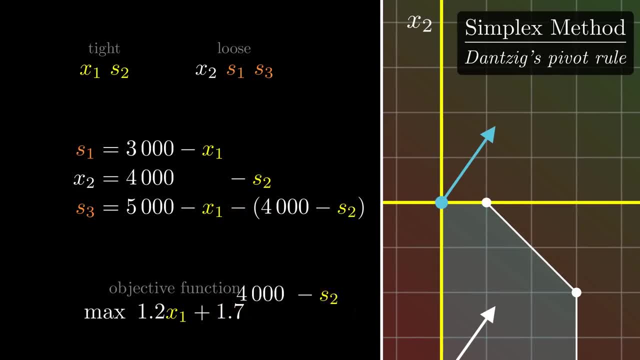 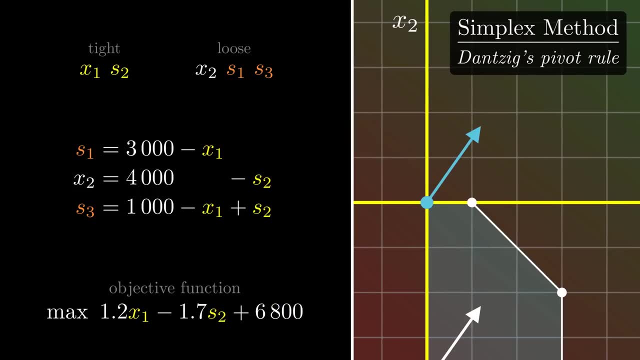 can now use as substitutes for the remaining x2s. After simplifying, we have successfully completed the pivot. As a sanity check, we see that setting the tight variables to zero again determines the vertex we're in, with the objective function's value increasing to 6800. 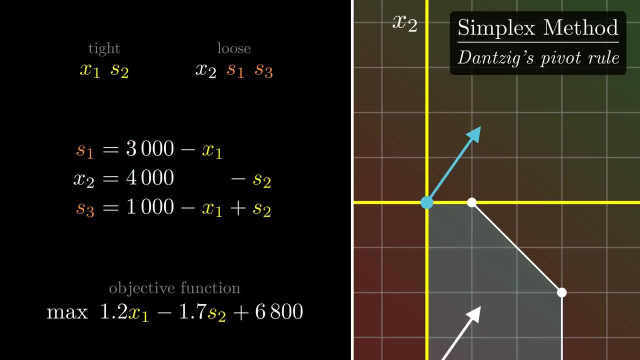 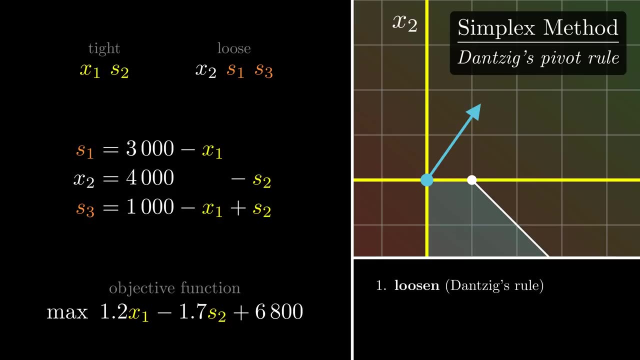 At this point, I highly urge you to pause the video and do the next pivot yourself, since it's a great way of checking how well you understand the algorithm. To help you out a bit, here are the steps you need to take. First, loosen a variable using Densik's pivot rule. Second, tighten a variable given the 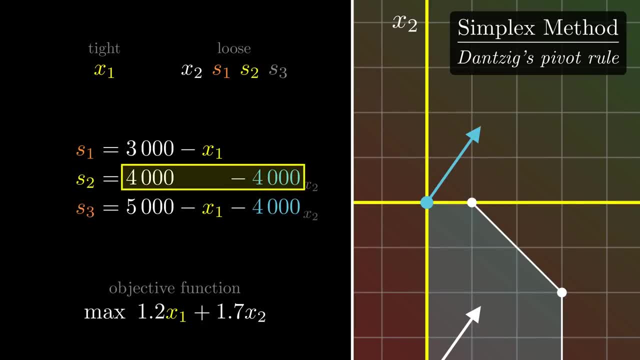 which brings out the constant value for the second equality, making s2 tight. Now, if we were to go further, s2 would have to go negative for the equality to still work, which is not allowed, since all variables have to be non-negative. 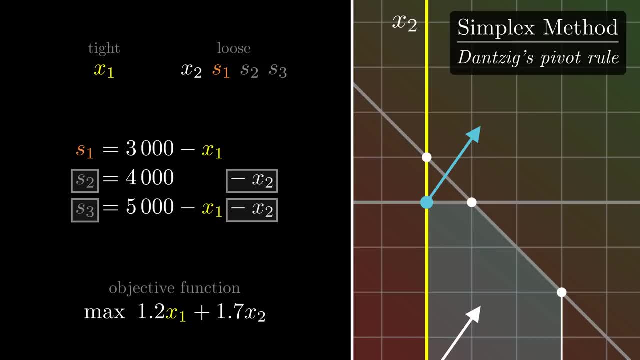 So, in other words, to calculate which variable to tighten, we're interested in the ratio between x2 and the constants. The larger it is, the sooner we reach it And, as we've seen, it is indeed s2, which we tighten. 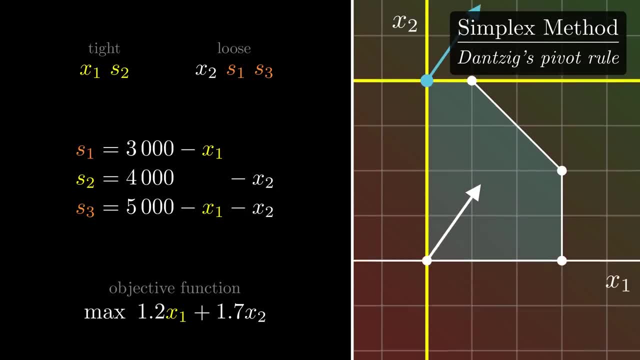 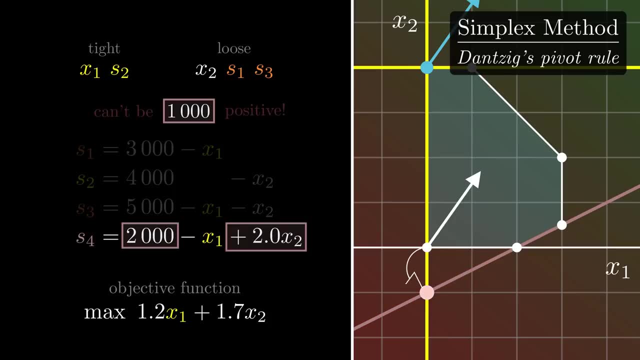 Note that if it's greater than zero, for example, if we had another equality like this one, we wouldn't want it, since increasing x2 in this case will never zero out the constant, since it's in the opposite direction. So what we actually want is the largest non-positive ratio. 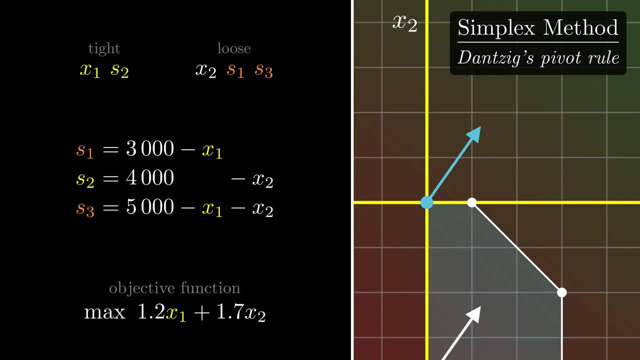 Now that we've loosened x2 and tightened s2,, we still have to fix the equalities and the objective function. Remember that loose variables belong only on the left side, which now isn't the case, As you can see by the highlighted s2s and x2s. 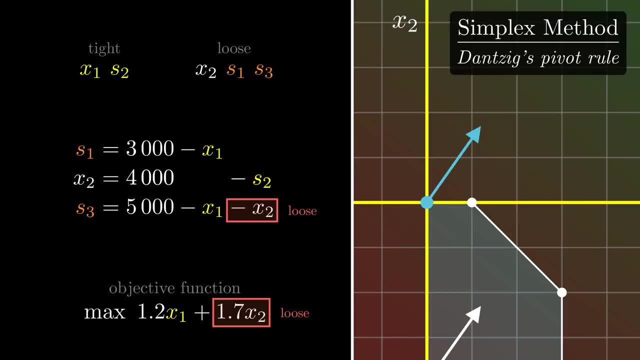 Swapping them solves the problem for the second equality, which we can now use as substitutes for the remaining x2s. After simplifying, we have successfully completed the pivot. As a sanity check, we see that setting the tight variables to zero again determines the vertex. 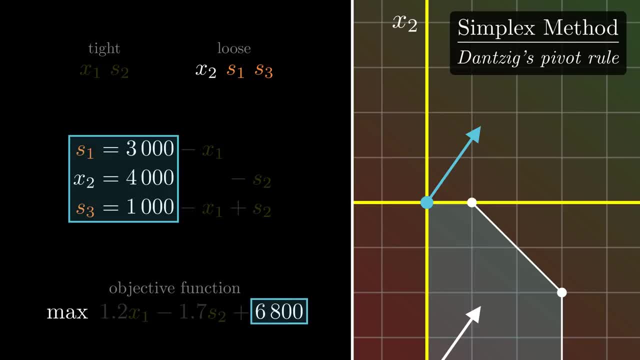 we're in, with the objective function's value increasing to 6800.. I highly urge you to pause the video and do the next pivot yourself, since it's a great way of checking how well you understand the algorithm. To help you out a bit, here are the steps you need to take. 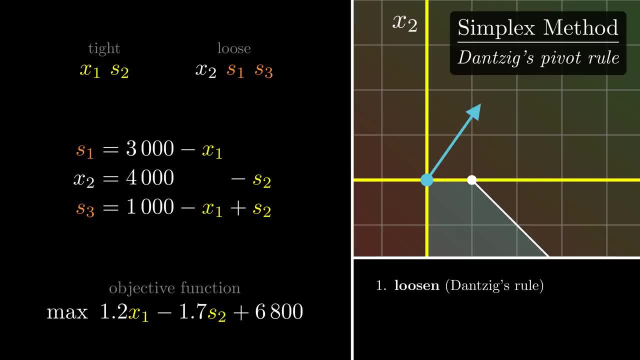 First, loosen a variable using DenseX Pivot Rule. Second, tighten a variable given the largest non-positive ratio And finally, fix the equalities by swapping and substituting. Okay, for the next pivot, we repeat exactly what we did for the first one. 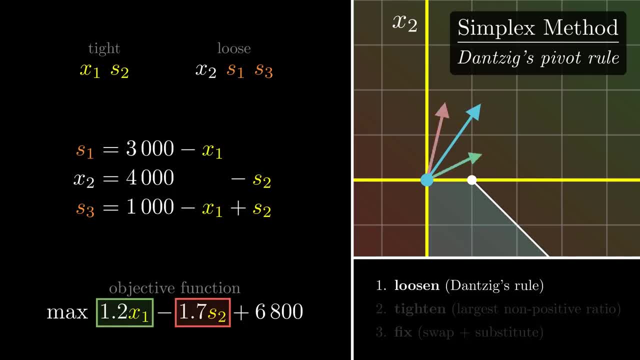 We determine the variable to loosen by the largest positive coefficient in the objective function, which is x1. We look at where x1 appears in the equalities and compare the ratios. The largest non-positive one corresponds to s3, which we tighten. 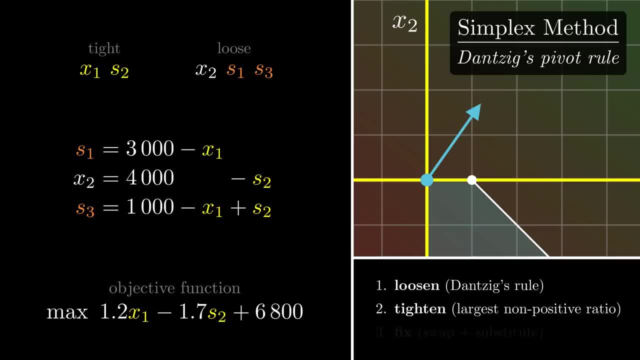 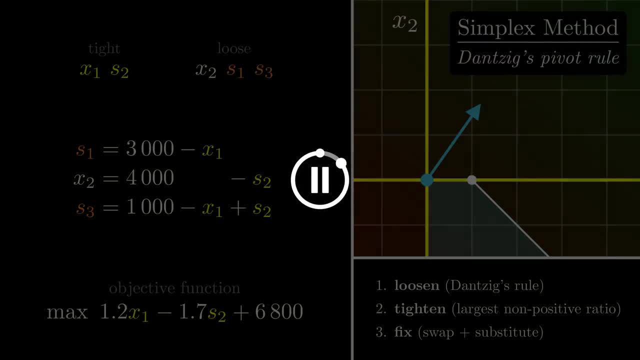 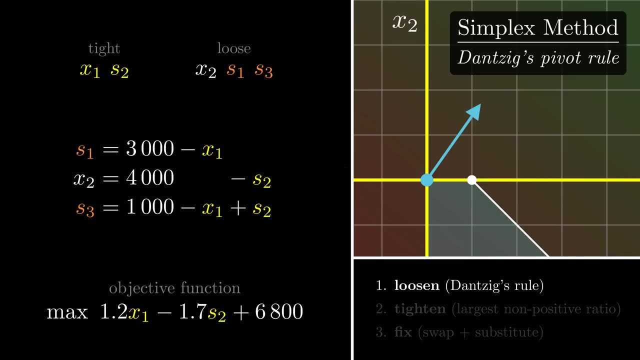 largest non-positive ratio And finally fix the equalities by swapping and substituting. Okay. for the next pivot, we repeat exactly what we did for the first one: We determine the variable to loosen by the largest positive coefficient in the objective function, which is x1.. 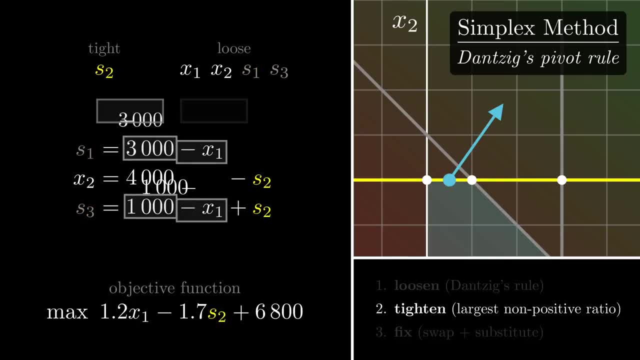 We look at where x1 appears in the equalities and compare the ratios. The largest non-positive one corresponds to s3, which we tighten. and finally, we fix the equalities in the objective function such that the loose variables are only on the left side. 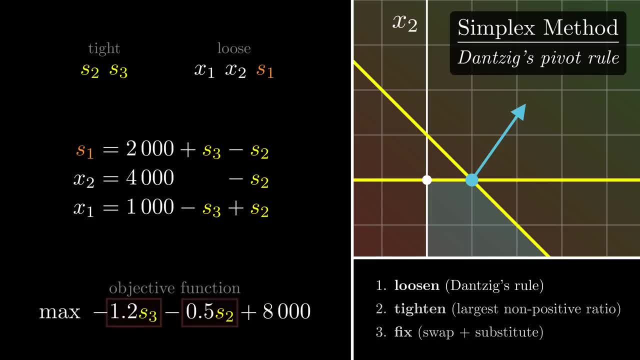 And we're done. We can see this because all of the coefficients of the objective function are now negative, so we can't improve any further. The optimum is 8000,, again achieved by setting x1 to 1000 and x2 to 4000,, which is the same as the. 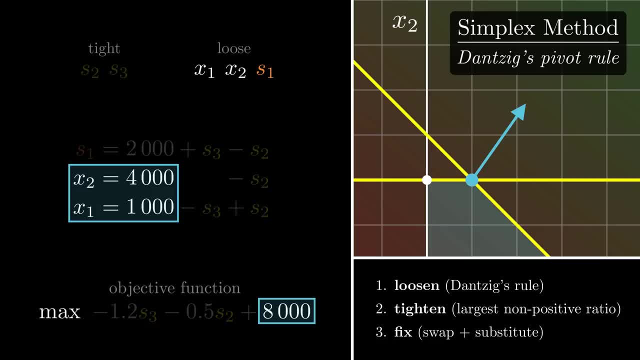 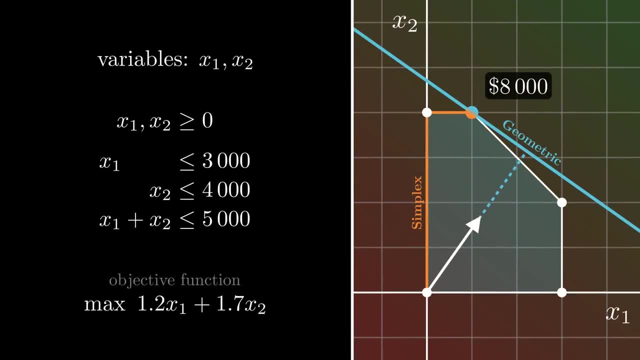 one from our geometric solution, which is a good indicator that the algorithm works as intended. So at this point we have solved the problem both geometrically and algorithmically, but it would be worth looking for more information in the next video. See you next time. 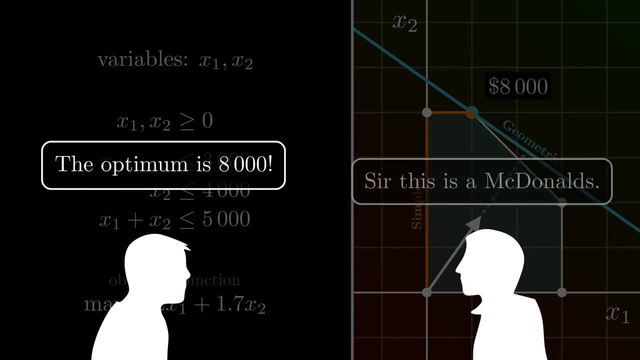 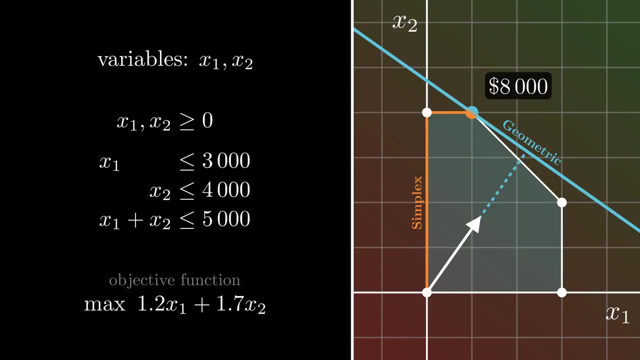 pretty hard to convince someone else that we did if we were to just show them the result. It would be nice if we could prove that the solution we found is truly optimal. One thing that comes to mind is combining the inequalities in a way that creates an upper bound on the objective function, because that would 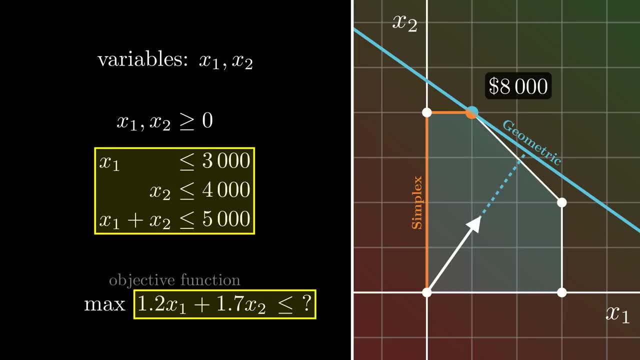 show that we literally cannot get a better result. As an example, if we multiply the first inequality by 1.2 and the second by 1.7 and we sum them up, we get that the objective function is less than or equal to 10,400, which 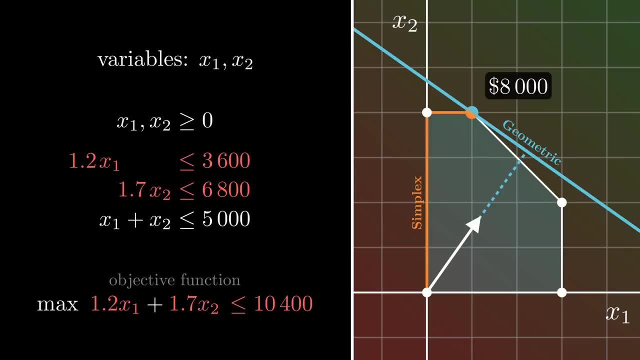 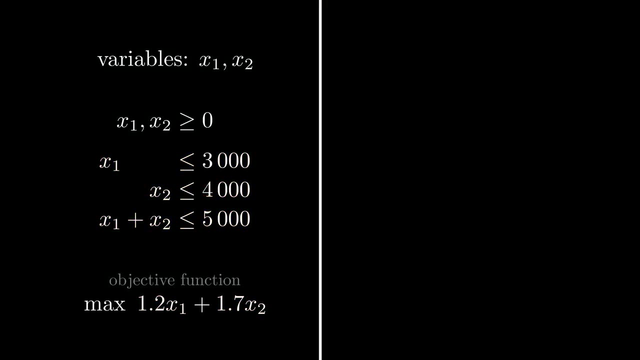 tells us that the objective function can never be greater than that. Or let's say, 0.2 times the first plus 0.7 times the second plus the third gives a better estimate of 8,400.. This looks promising. so let's formalize and turn these. 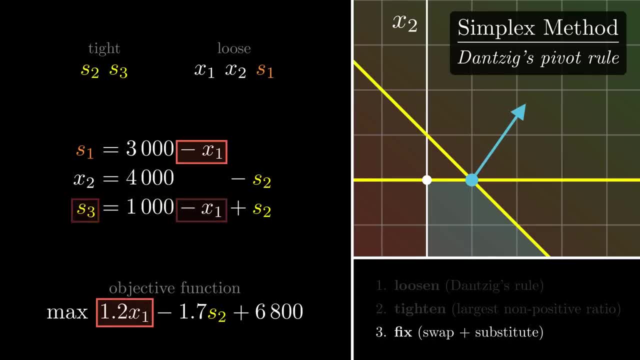 And finally we fix the equalities in the objective function such that the loose variables are only on the left side, And we're done. We can see this because all of the coefficients of the objective function are now negative, so we can't improve any further. 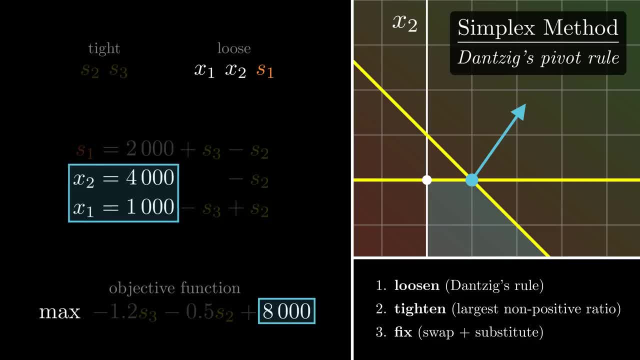 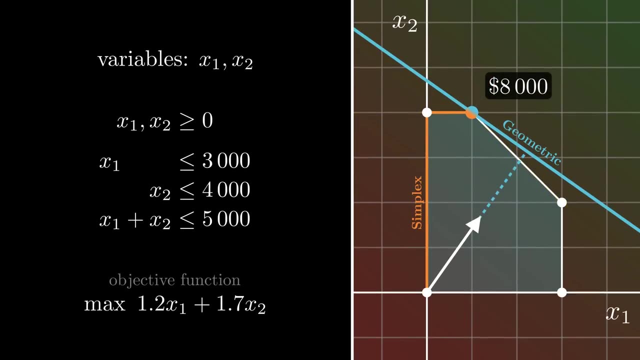 The optimum is 8000, again achieved by setting x1 to 1000 and x2 to 4000,, which is the same as the one from our geometric solution, which is a good indicator that the algorithm works as intended. So at this point we have solved the problem both geometrically and algorithmically. 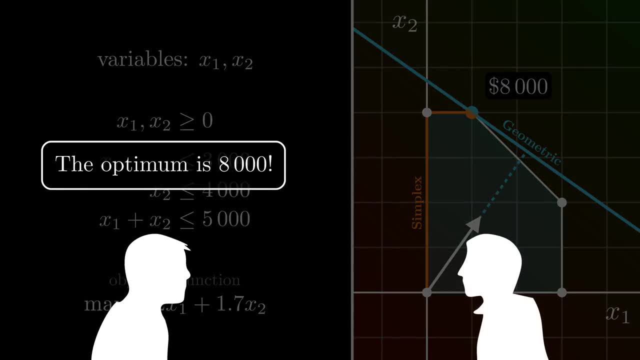 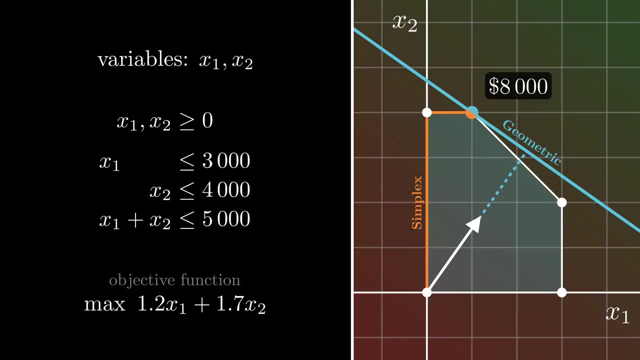 but it would be pretty hard to convince someone else that we did, if we weren't doing it, If we were to just show them the result. It would be nice if we could prove that the solution we found is truly optimal. One thing that comes to mind is combining the inequalities in a way. 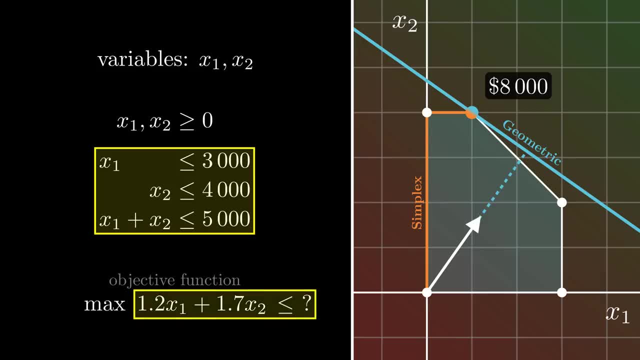 that creates an upper bound on the objective function, because that would show that we literally cannot get a better result. As an example, if we multiply the first inequality by 1.2 and the second by 1.7, and we sum them up, we get that the objective function is less than or equal to 10400.. 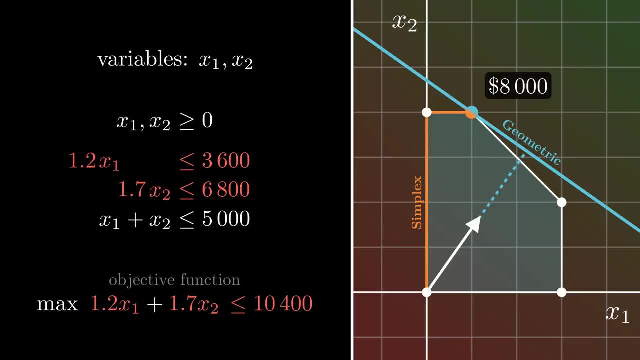 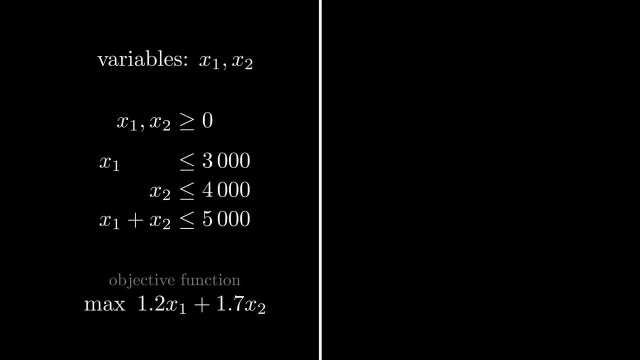 Which tells us that the objective function can never be greater than that. Or let's say 0.2 times the first plus 0.7 times the second plus the third gives a better estimate of 8400.. This looks promising. so let's formalize and turn these numbers into variables. 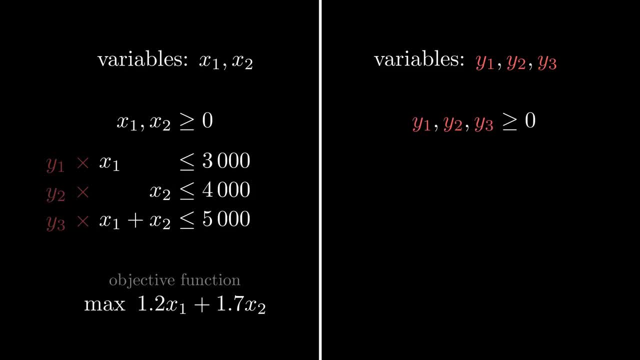 They have to be non-negative, otherwise the inequality flips, and must be set in such a way that the left side is at least the objective function. Since we want to constrain it Finally, we want to minimize the right side and we just created a linear program. 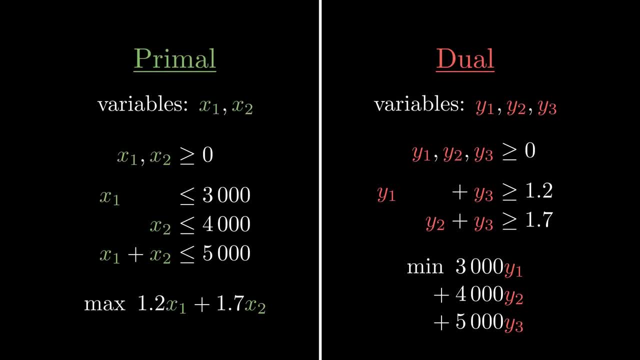 This is called the dual linear program and is, in my opinion, perhaps the most beautiful thing about linear programming. The dual bounds our original linear program, which we'll call the primal from now on, and vice versa. Solutions to the primal will always be less than or equal to. 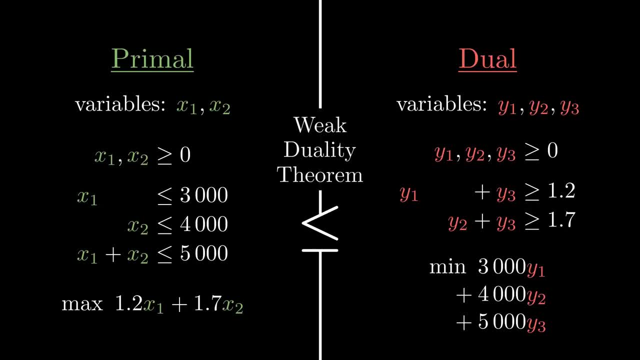 the solutions of the dual, and this is referred to as the weak duality theorem. Now, this is not quite what we had in mind. We actually wanted an equality, because only then would we be able to confirm that the solution we found is truly the optimum. 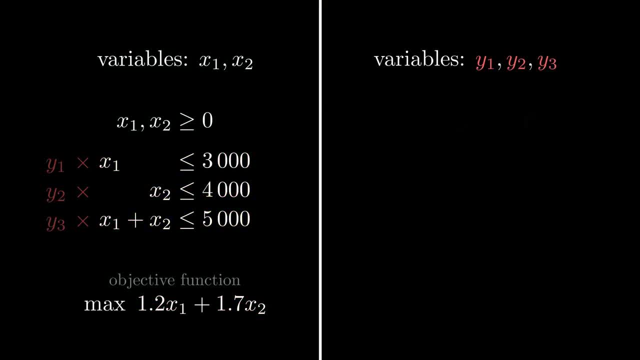 numbers into variables. They have to be non-negative, otherwise the inequality flips, And must be set in such a way that the left side is at least the objective function. since we want to constrain it Finally, we want to minimize the right side and we just created a linear program. This is called the dual linear. 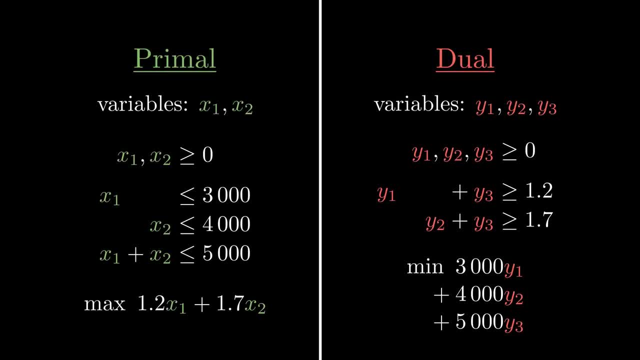 program and is, in my opinion, perhaps the most beautiful thing about linear programming. The dual bounds, our original linear program, which we'll call the primal from now on, and vice versa. Solutions to the primal will always be less than or equal to 0.2 times the original linear program, and vice versa. 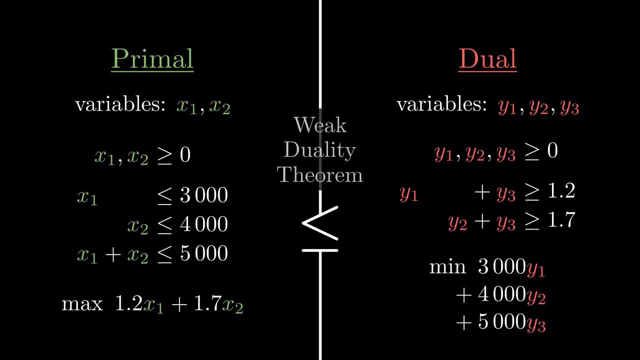 Now, this is not quite what we had in mind. We actually wanted an equality, because only then would we be able to confirm that the solution we found is truly the optimum. This is referred to as the strong duality theorem and, incredibly, if the primal has an optimum, it holds true, meaning that we can always 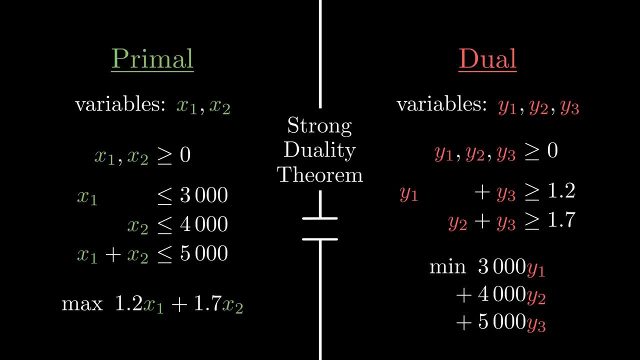 find the proof that we were looking for. Besides proving that the solution is true, this is done usingίο whichtım τους путnhehely To prove it's proven optimality. duality has a number of other interesting uses, which are sadly beyond. 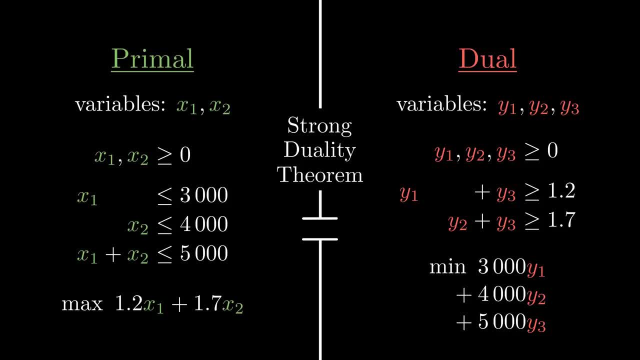 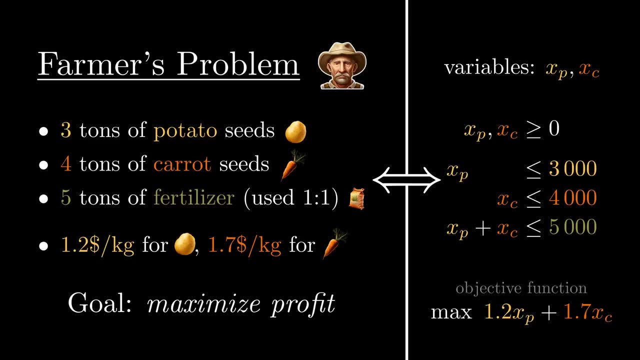 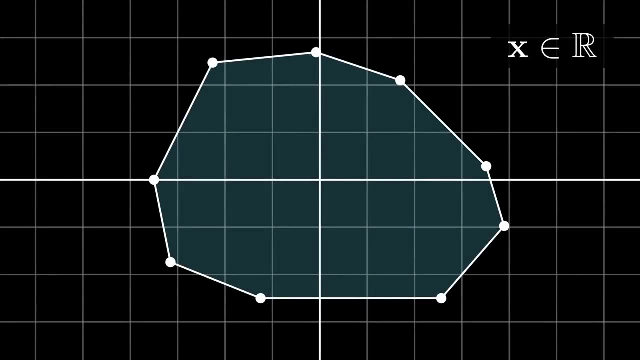 the scope of this video, but will likely be in the next one. It's now safe to say that we've thoroughly covered the farmers problem, but it turns out that we were actually pretty lucky When formulating the problem. we decided that the variables are real numbers, since planting a 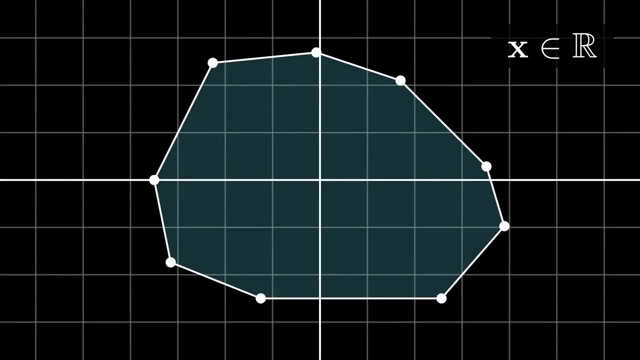 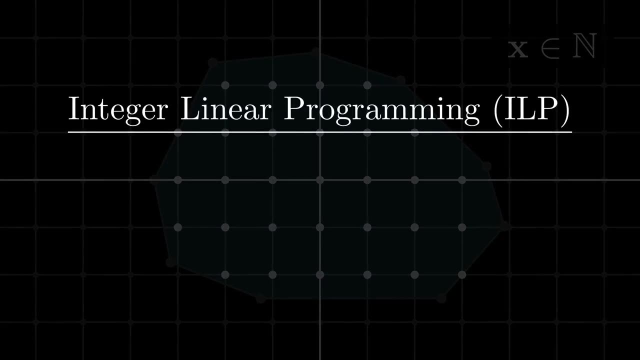 fraction of a kilogram makes sense. However, imagine that the things we wanted to plant were trees, Numer Favorites. In that case, we would like to restrict the solutions to integers only, since planting a portion of a tree is difficult. This is referred to as integer linear programming, or ILP for short, and it naturally poses two. 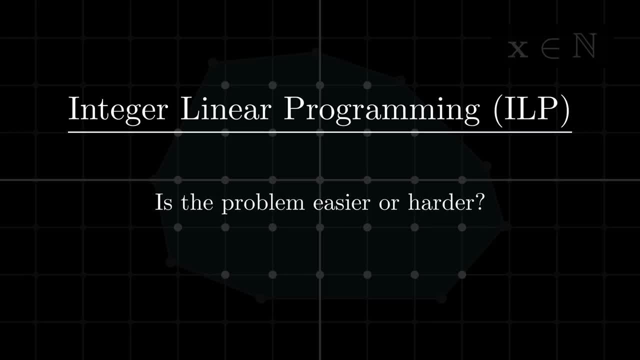 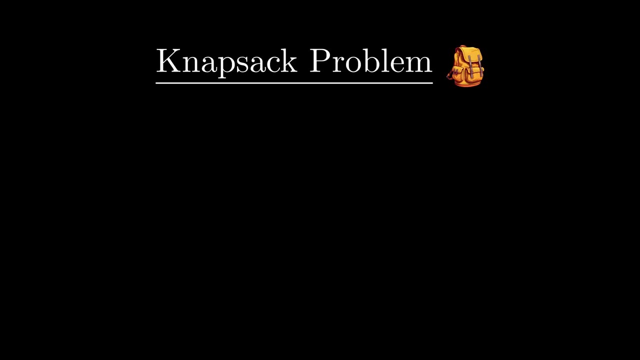 questions: Is the problem easier or harder than linear programming, And can we still solve it efficiently? Well, to illustrate that it gets a whole lot harder, we'll formulate the Knapsack problem, an infamous NP-hard problem, as an integer linear program. 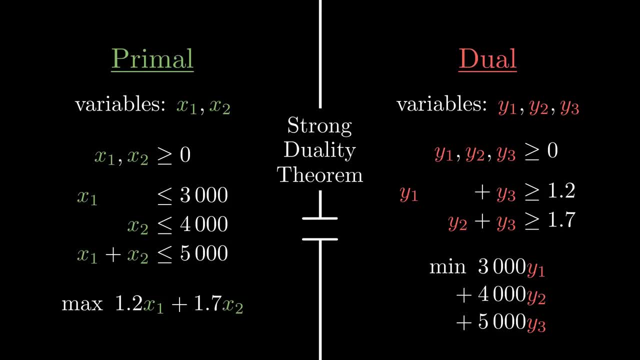 This is referred to as the strong duality theorem and, incredibly, if the primal has an optimum, it holds true, meaning that we can always find the proof that we were looking for. Besides proving optimality, duality has a number of other interesting uses. 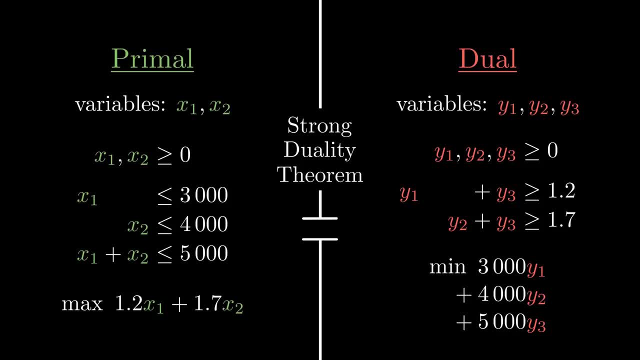 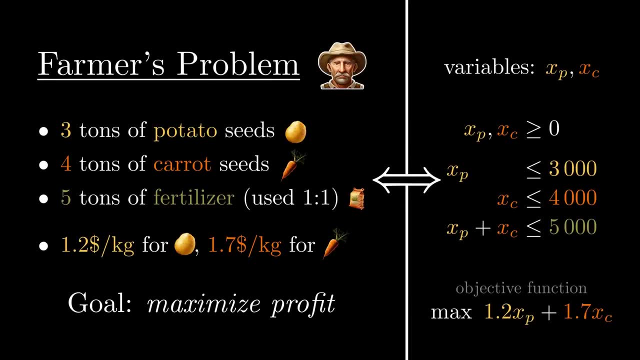 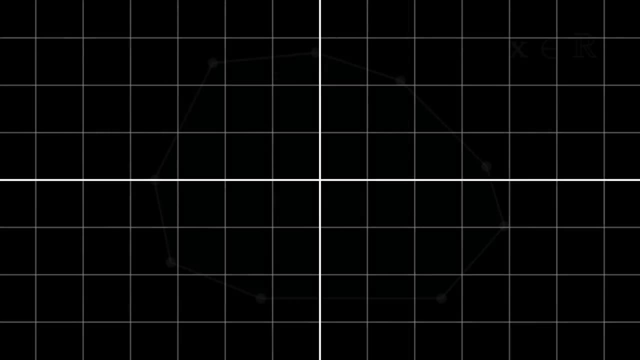 that are sadly beyond the scope of this video. So let's get started. It's now safe to say that we've thoroughly covered the farmer's problem, but it turns out that we were actually pretty lucky When formulating the problem. we decided that the variables are real numbers, since planting a fraction of a kilogram makes 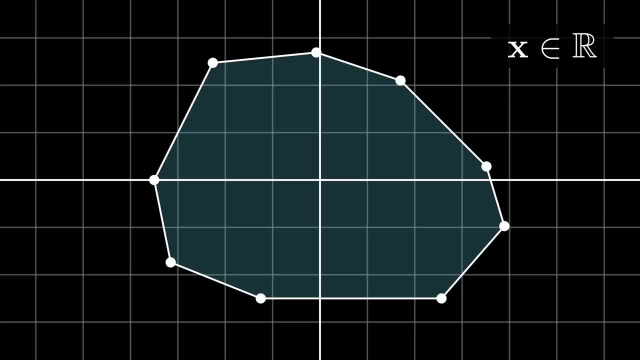 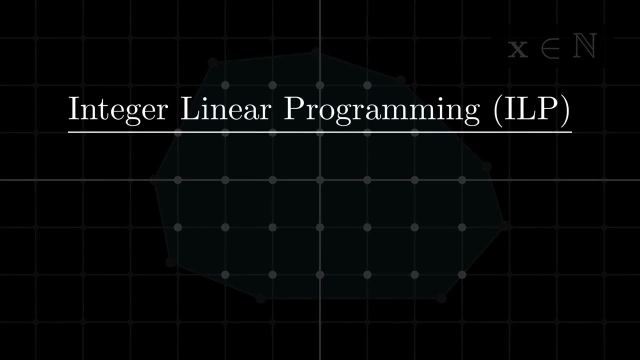 sense. However, imagine that the things we wanted to plant were trees. In that case, we would like to restrict the solutions to integers only, since planting a portion of a tree would be difficult. This is referred to as integer linear programming, or ILP for short. 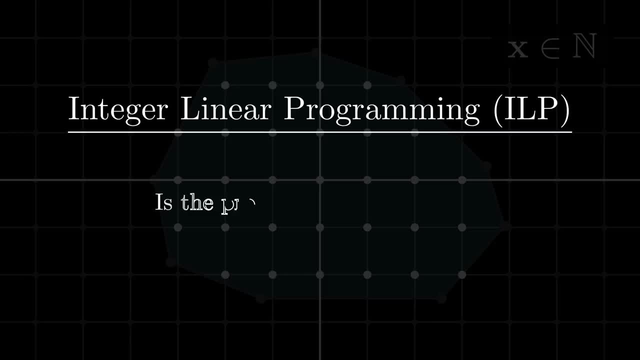 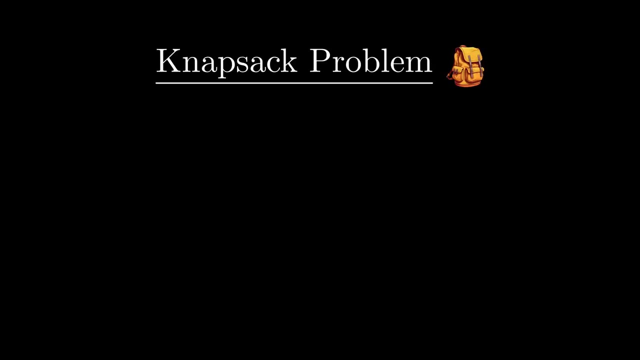 and it naturally poses two questions: Is the problem easier or harder than linear programming, and can we still solve it efficiently? Well, to illustrate that it gets a whole lot harder, we'll formulate the knapsack problem- an infamous NP-hard problem- as an integer linear program. The task is this: We're given n items. 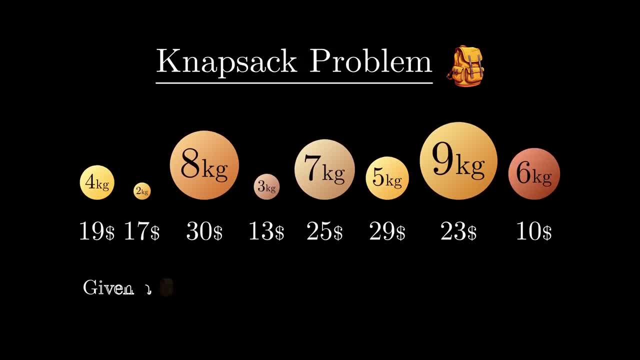 a weight and a price. Given a backpack with a carry weight, say, 17 kilograms, our task is to maximize the price of the items we take without exceeding the carry weight. For this problem, using binary variables will be very helpful. 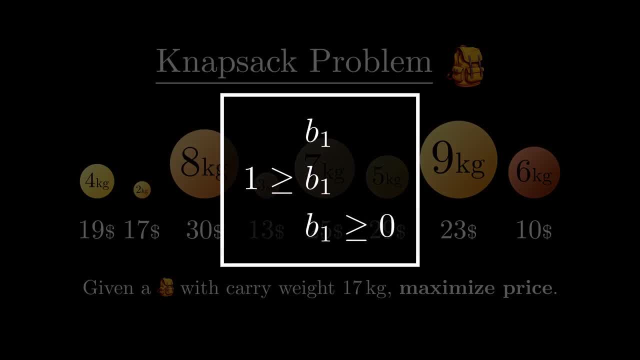 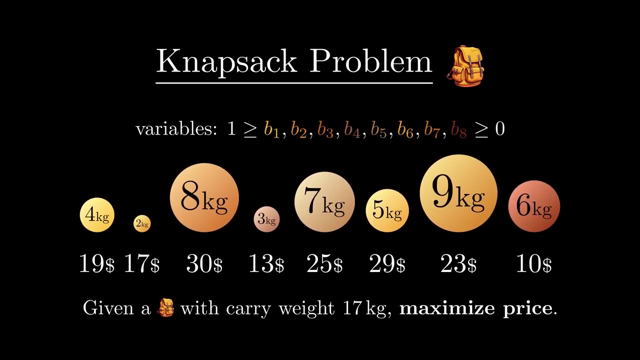 We can achieve this by creating a variable and adding inequalities such that its value is between 0 and 1.. Since it's an integer linear program, the only values the variable can have will therefore be 0 and 1.. There will be one binary variable for each item. 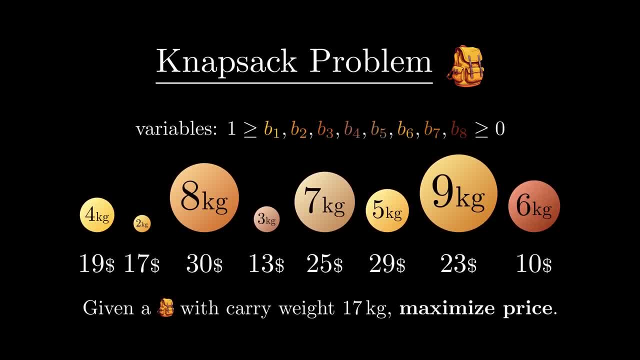 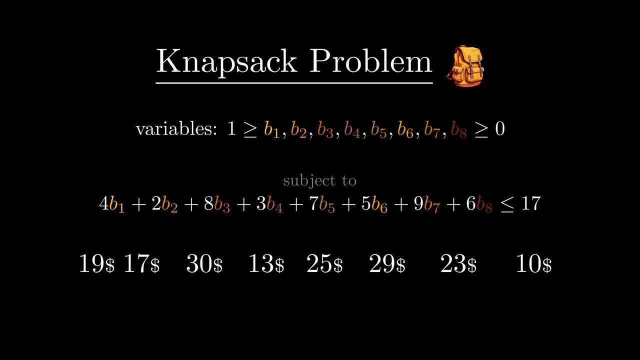 having value 1 if we take it and 0 if we don't, There will only be one additional inequality, which is that the weight of the items we carry doesn't exceed the backpack's carry weight. This can be done by multiplying the binary variables with their weights. 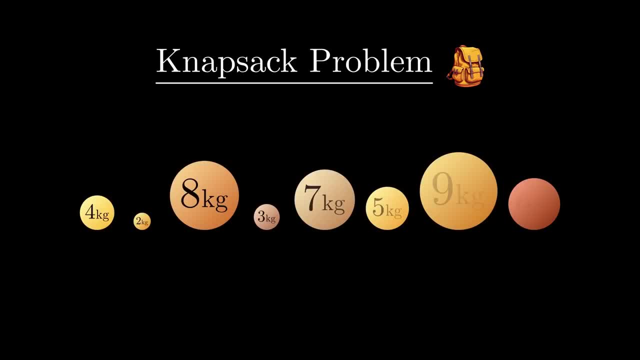 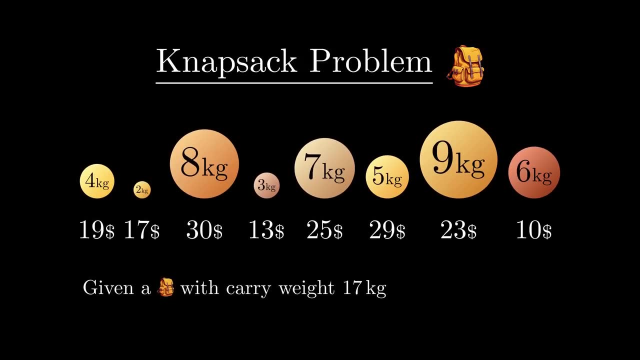 The task is this: We're given n items, each having a weight and a price. Given a backpack with a carry weight, say 17 kilograms, our task is to maximize the price of the items we take without exceeding the carry weight. 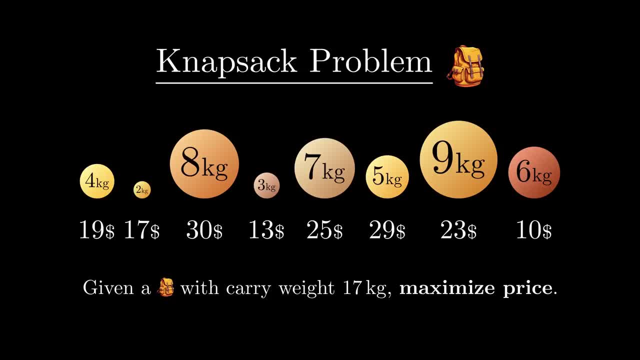 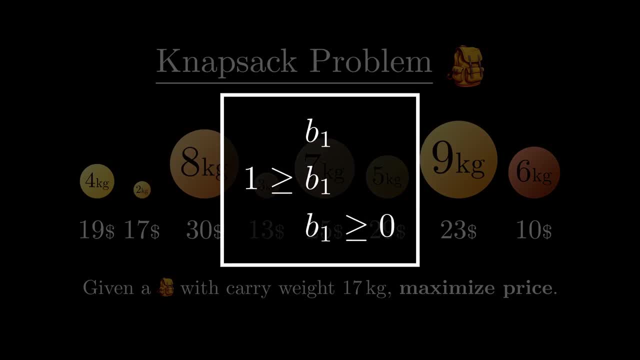 For this problem, using binary variables will be very helpful. We can achieve this by creating a variable and adding inequalities such that its value is between 0 and 1.. Since it's an integer linear program, the only values the variable can have will therefore. 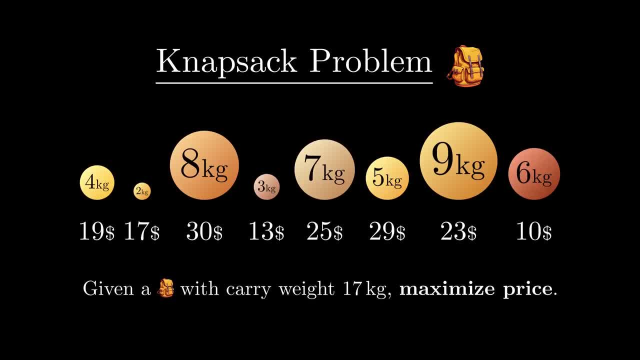 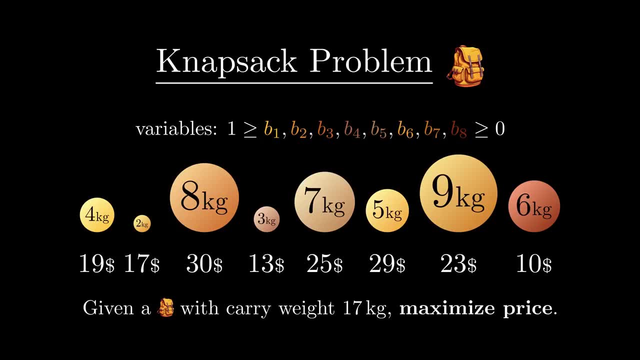 be 0 and 1.. There will be one binary variable for each item having value 1 if we take it and 0 if we don't. There will only be one additional inequality, which is that the weight of the items we carry. 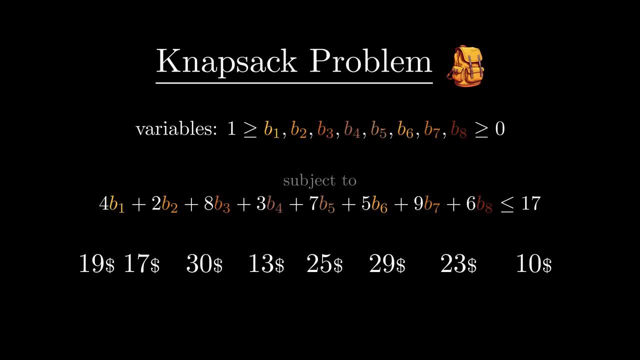 doesn't exceed the backpack's carry weight. This can be done by multiplying the binary variables with their weights. If the item is not taken, its variable will be 0, and its weight won't be counted, otherwise it will be. Similarly, the function to maximize is the price of the items we carry, again done by: 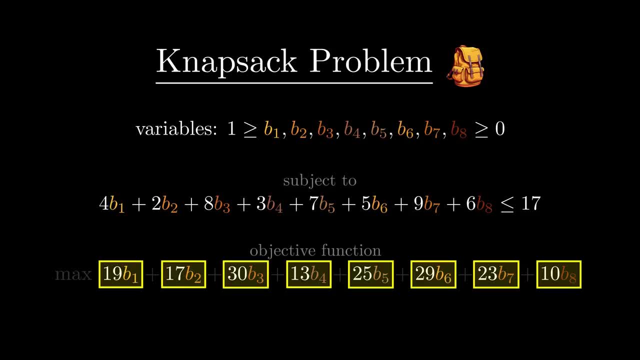 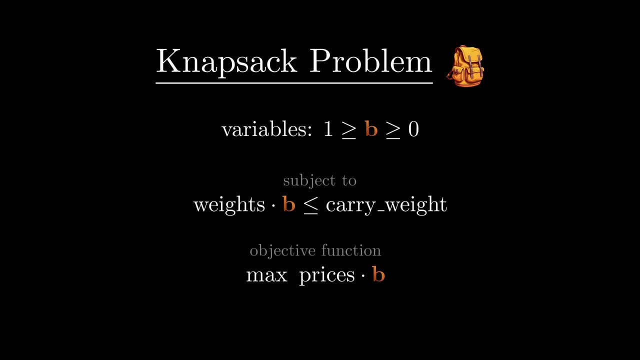 multiplying the binary variables with their prices. Alternatively, if we put the variables into a vector, the linear program can be stated like this, which is quite a bit more concise: And since there's been enough theory, let's write something else. Let's write something else. 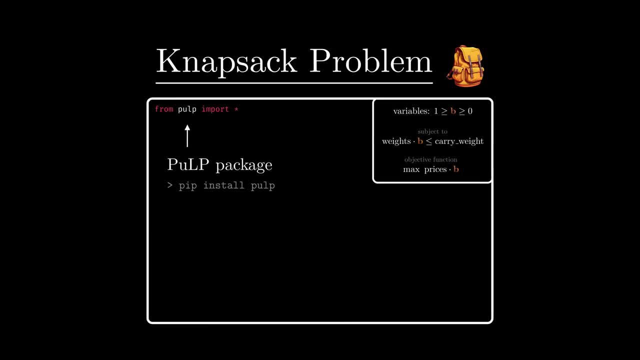 Let's write some Python code that solves this problem, using the pull package, which is an excellent tool for formulating and solving linear programs of all shapes and sizes. Taking the data from the example we've seen, we'll formulate the variables, the single. 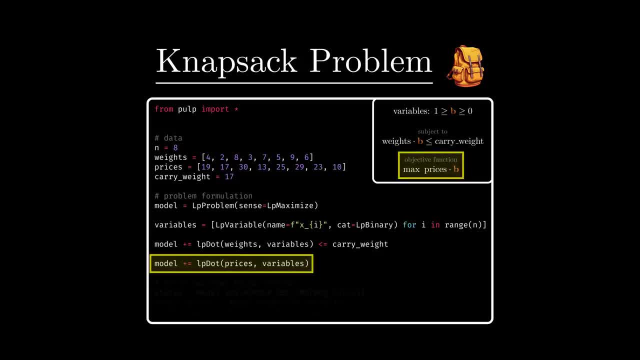 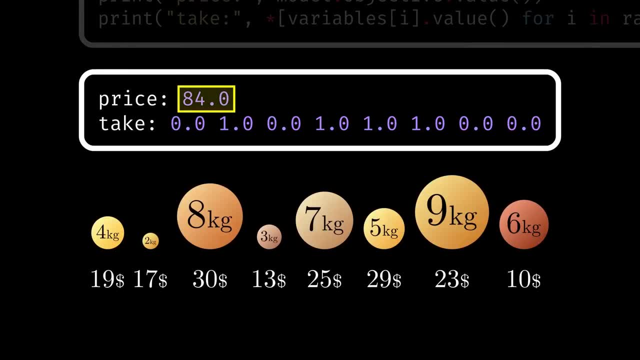 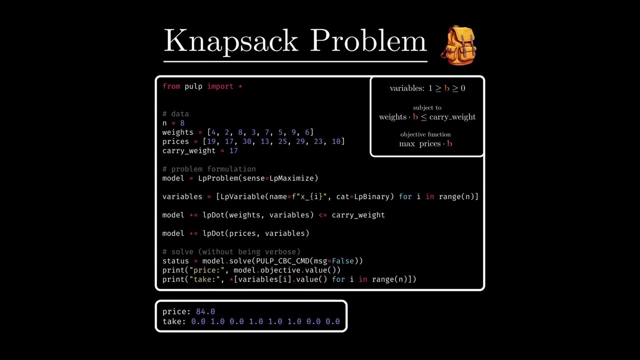 inequality, the objective function and finally solve the problem Printing the output. the optimal price of the items in this case is 84, if we take items 2,, 4,, 5, and 6.. So, while the problem is still NP-hard, there is a significant amount of optimizations that. 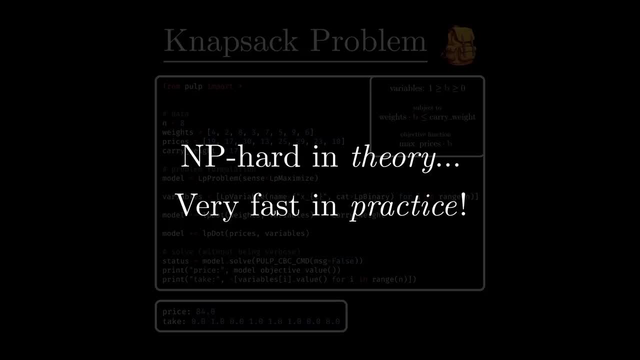 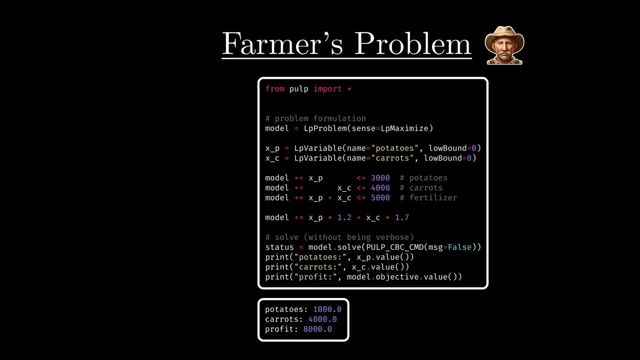 the solver can do, which makes it run very fast on real-world data and likely much faster compared to whatever program you and I can write. As another pulp example, this is an implementation of the farmer's problem that we saw earlier in the video. 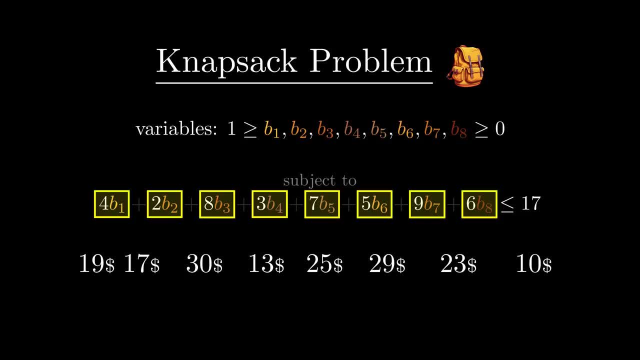 If the item is not taken, its variable will be 0, and its weight won't be counted, Otherwise it will be. Similarly, the function to maximize is the price of the items we carry, Again done by multiplying the binary variables with their prices. 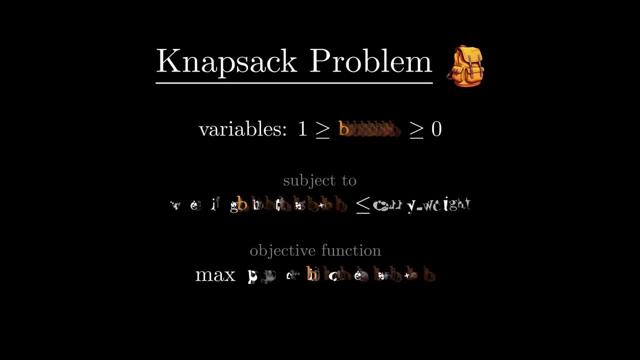 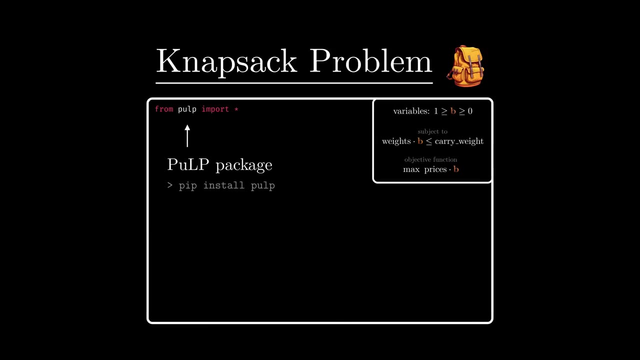 Alternatively, if we put the variables into a vector, the linear program can be stated like this, which is quite a bit more concise, And since there's been enough theory, let's write some Python code that solves this problem, using the pull package, which is an excellent tool for formulating and solving linear programs of all. 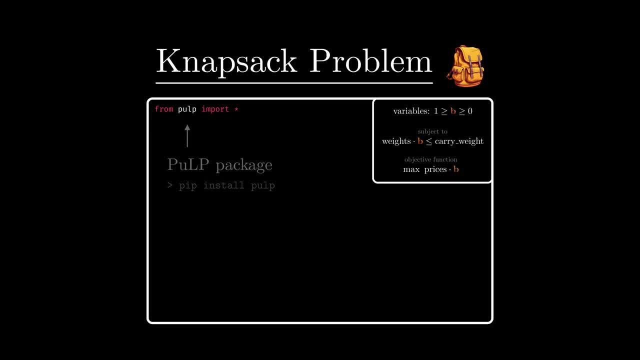 shapes and sizes. If you're interested in learning more about linear programming, please subscribe to our channel and don't forget to hit the bell button if you haven't already, so you don't miss any of our new videos. Taking the data from the example we've seen, we'll formulate the variables. 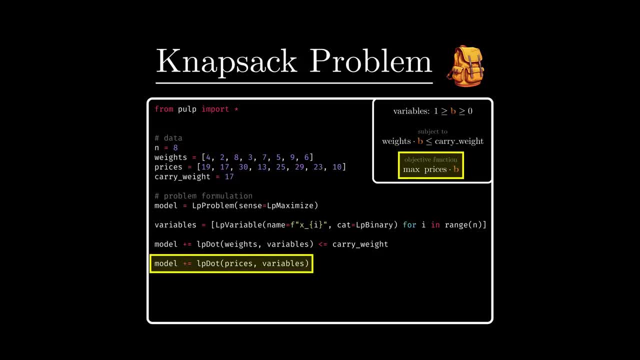 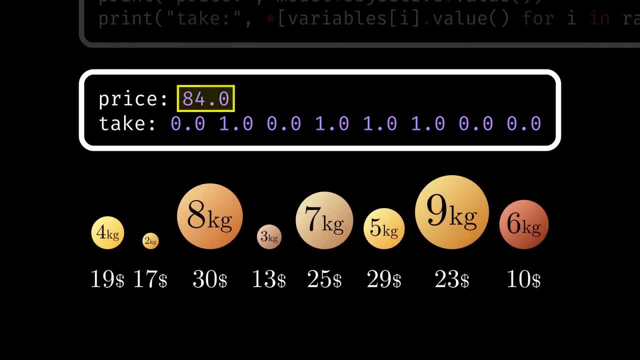 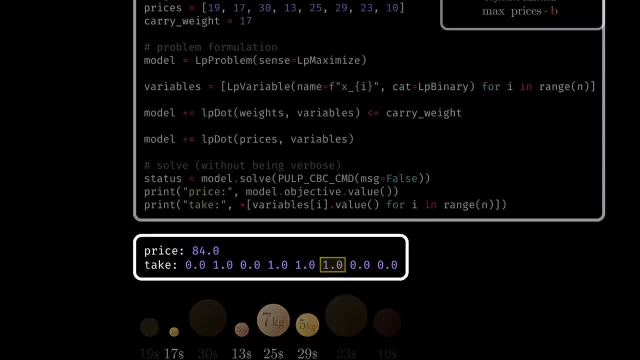 the single inequality, the objective function and finally solve the problem Printing the output. the optimal price of the items in this case is 84, if we take items 2,, 4,, 5, and 6.. So, while the problem is still NP-hard, there is a significant amount of optimizations that the 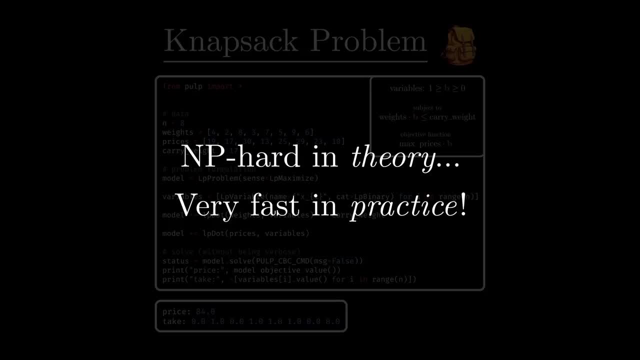 solver can do. The problem is still NP-hard. there is a significant amount of optimizations that the solver can do. So, while the problem is still NP-hard, there is a significant amount of optimizations that the solver can do, Which makes it run very fast on real-world data and likely much faster compared to whatever program. 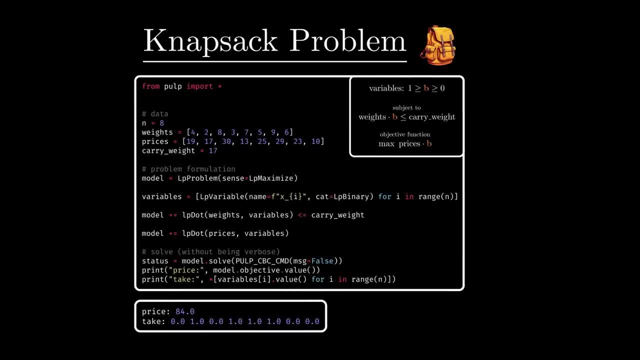 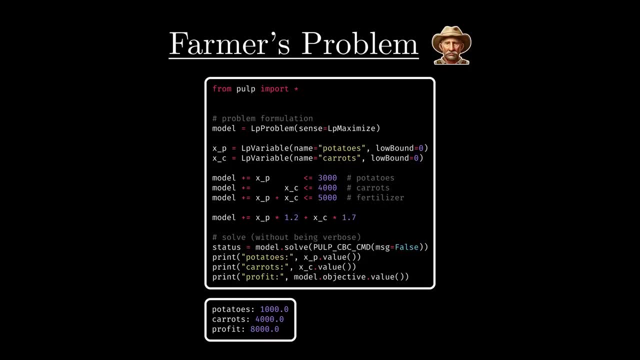 you and I can write As another pulp example, this is an implementation of the farmer's problem that we saw earlier in the video. I have to say that solving the problem we spent the majority of the video on, in 20 lines of code and a fraction of a second, feels pretty satisfying. There are many. 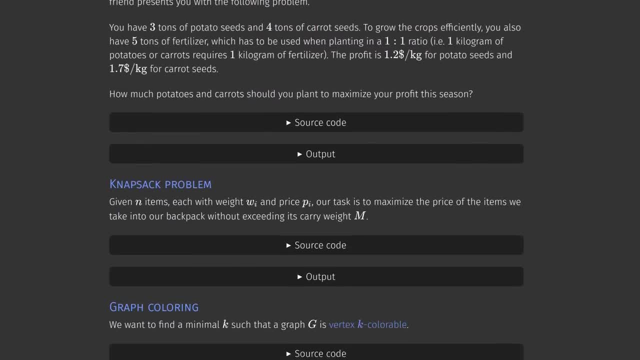 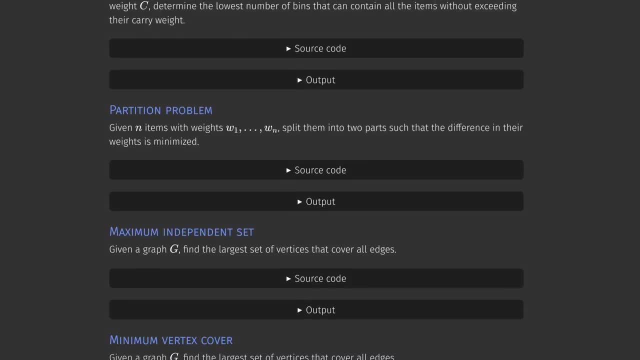 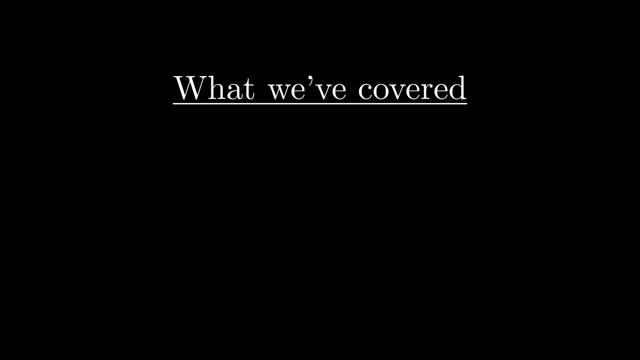 more examples that can be solved with both regular and integer linear programming and, if you're interested, I left a link to my website showcasing the interesting ones in the description. So, as an introduction to linear programming, I think we've covered most of the important topics. 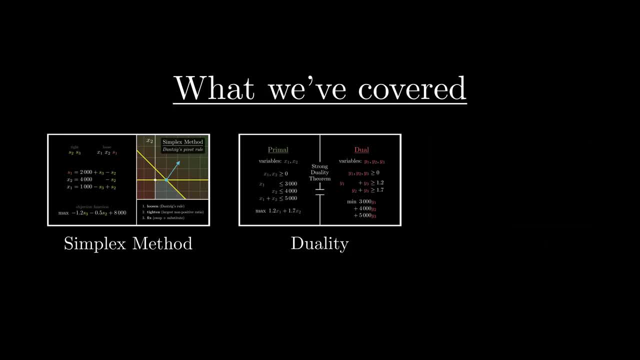 that being the simplex method, duality and integer linear programming. However, we've covered them rather superficially and there is a great deal of nuance to each of them. For the simplex method, what if isn't a vertex? How do we start?